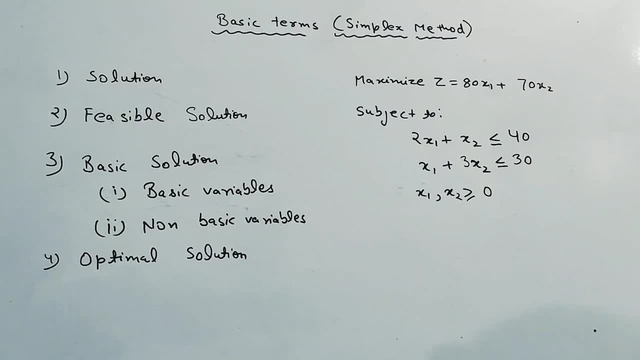 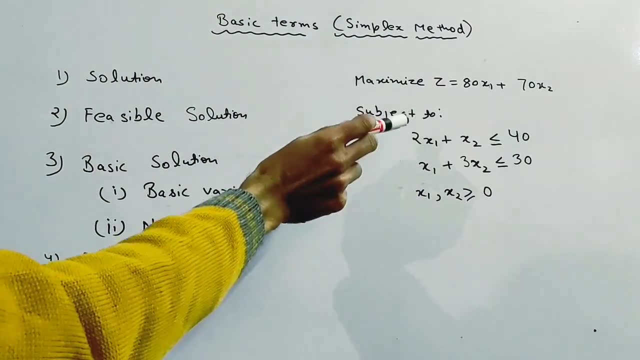 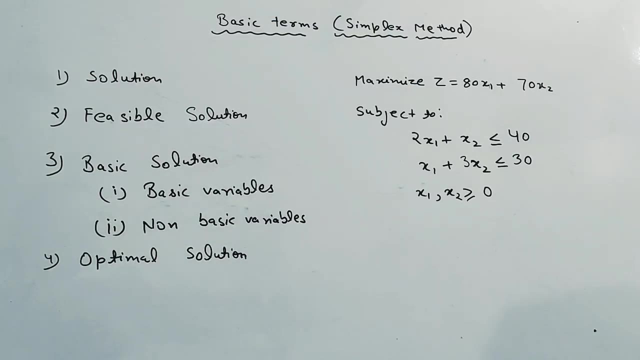 than or equal to 0.. So our first term is solution. Solution refers to decision variables ki wo saari values jo in constraints ko satisfy karti hai. Next is feasible solution. Feasible solution refers to decision variables ki wo saari values jo na sirf constraints ko satisfy. 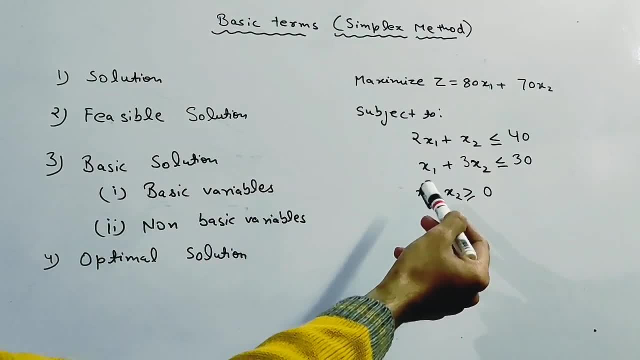 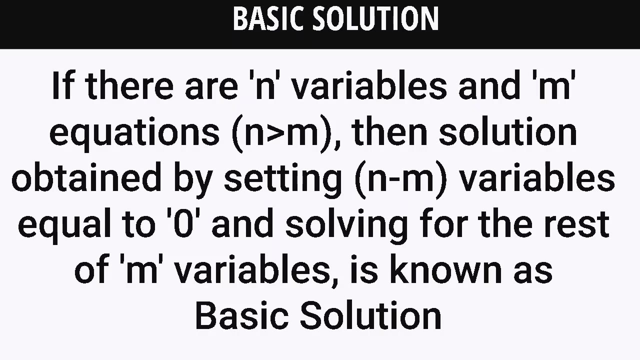 karti hai, Bal ki ye non-negativity constraint ko bhi satisfy karti hai. Third is basic solution. To understand basic solution, we must understand its definition. Suppose there are n number of variables and m number of equations. where n is greater than m, Then by putting n minus, 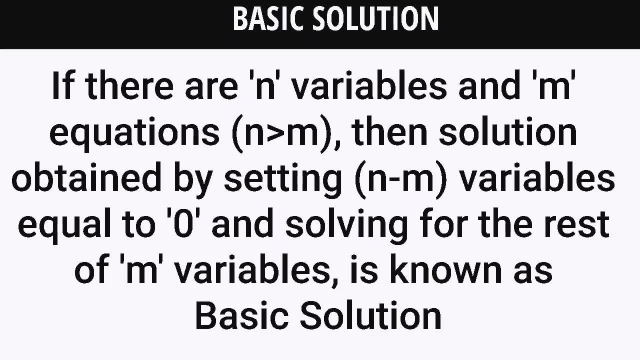 m variables equal to the 0 and solving the rest of the equations, the solution that we get is known as basic solution. n minus m variables- je ne hamne 0 rakha hai- are known as known basic variables. jab ki jo bachi gay m variables. these m variables are known as basic variables. For example suppose: 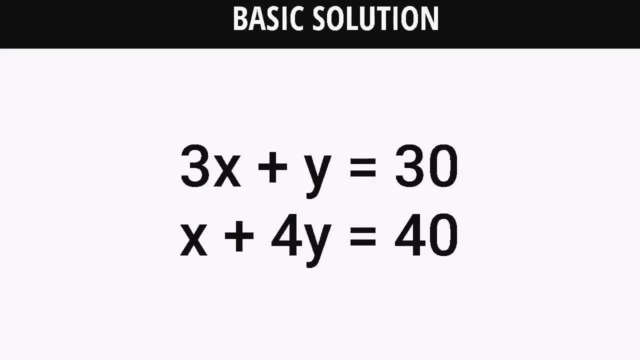 there are 2 equations: 3x plus y is equal to 30, x plus 4y is equal to 40.. Aap 2 equations hai, 2 variables hai. hame issa aasaani, se solve kar sakte hai by substitution, by elimination. 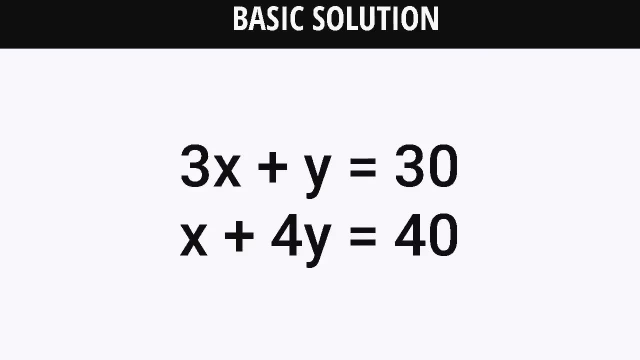 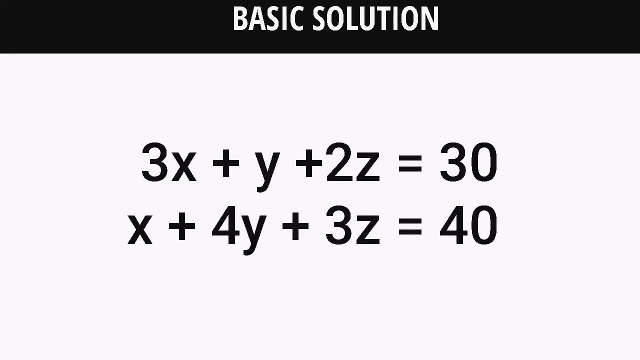 or by graphical method. But now suppose there are two variables. there are n minus n variables, which are known as basic variables. These n minus m variables are known as basic variables. For example, suppose two equations: 3x plus y plus 2z is equal to 30, and x plus 4y plus 3z is equal to 40.. 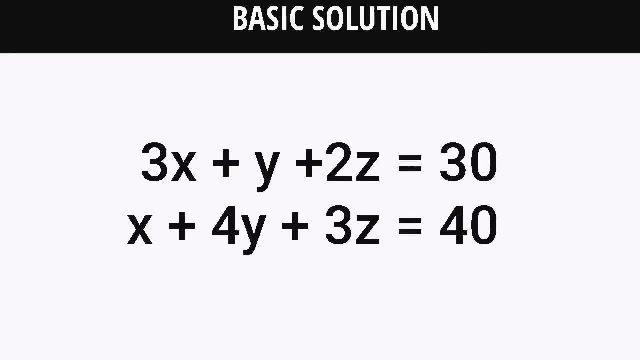 Now here there are three variables, but there are two equations. We cannot solve them with substitution or elimination method. There are three variables and two equations. It is very unfair. So we have to keep 3 minus 2, that is, one variable, as 0. After that we will have two. 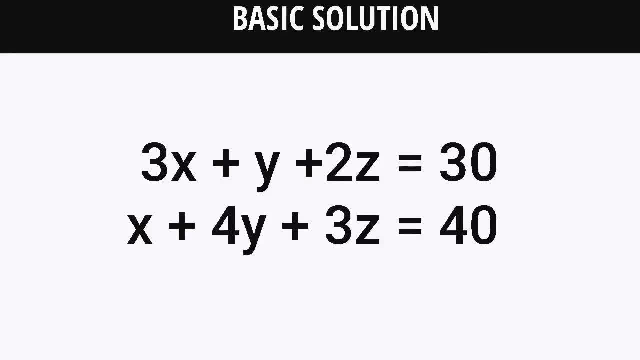 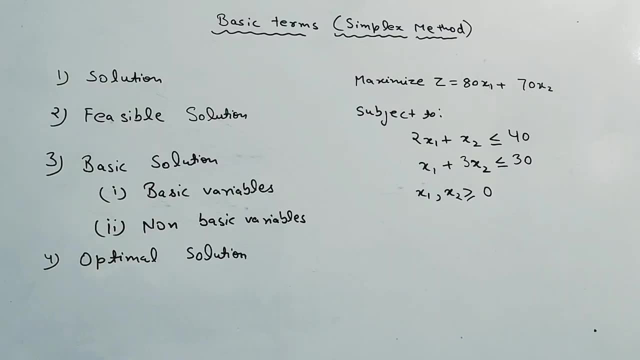 variables and two equations which we can solve easily. The variable which we keep as 0 will be our non-basic variable and the variables which will be left will be our basic variables. Finally, we have optimal solution. Optimal solution means all the values of decision variables which 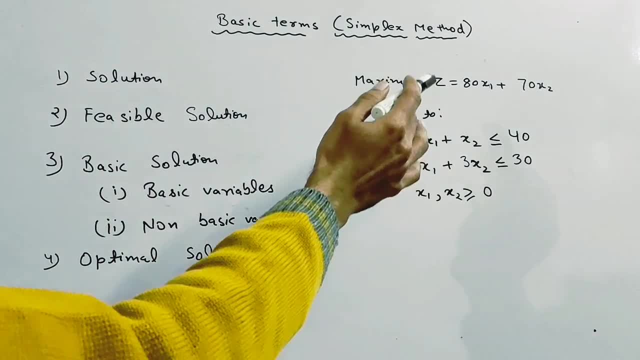 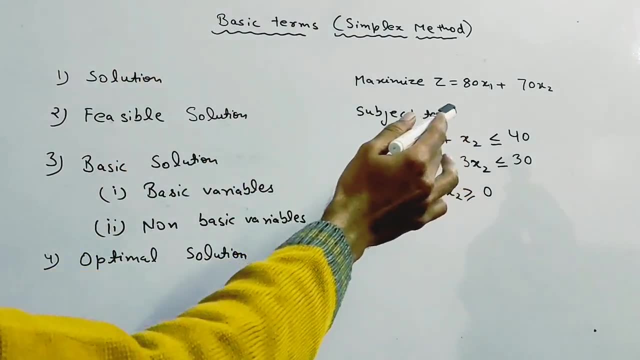 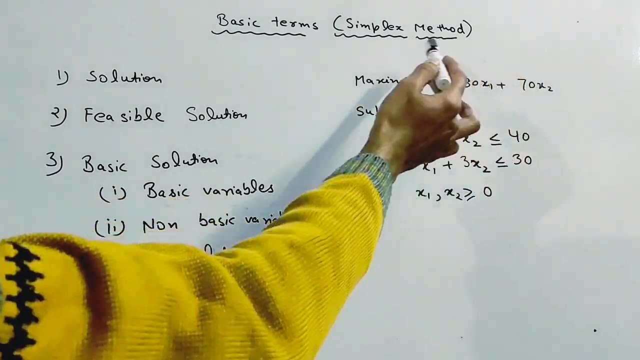 not only satisfy these constraints, but also optimize our objective function. For example, in this particular case, all the values of x1, x2, which are also satisfying these constraints, are also providing us the maximum value of our objective function. We can show this problem by 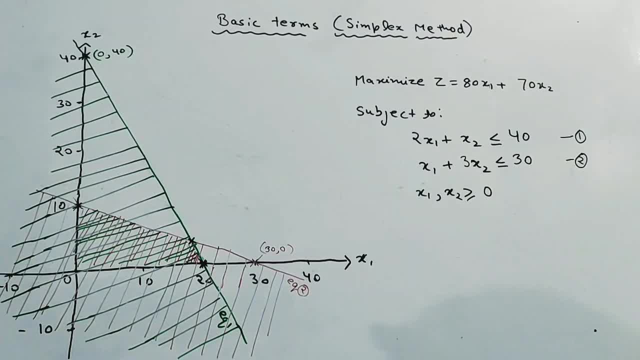 this graph. So first term is solution. Solution means all the values of decision variables which satisfy all the constraints. So graphically, we have given this solution region as common shaded region. So we have given this solution region as common shaded region. So graphically we have: 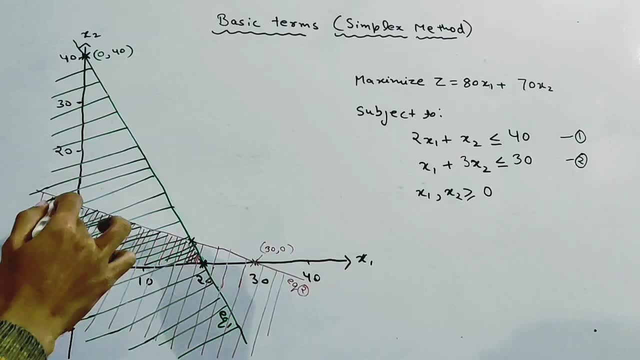 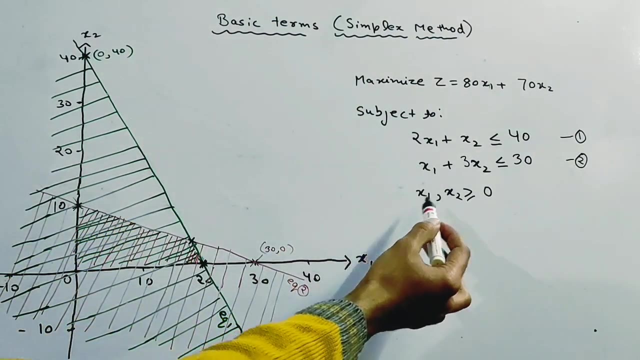 shown this solution region as common shaded region. So graphically we have shown this solution region as common shaded region. All these values which are in this common shaded region satisfy these two constraints. Next is feasible solution. Feasible solution means all the values of decision variables which not only satisfy these constraints but also satisfy non-negativity constraints. 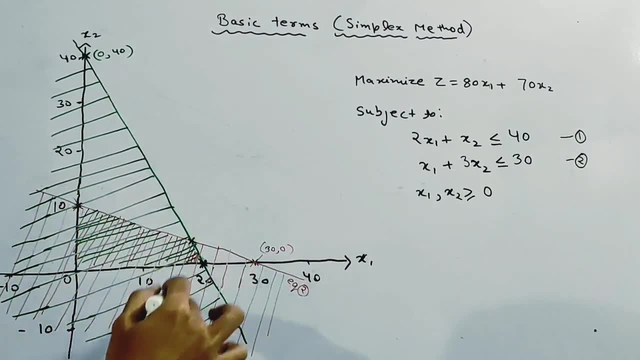 So, graphically speaking, the part of common shaded region which is in first quadrant or which is in the right side of 0. that is this part. This part is known as feasible region and all the values in this feasible region are known as feasible solution. Next is basic solution. Graphically: basic solution. 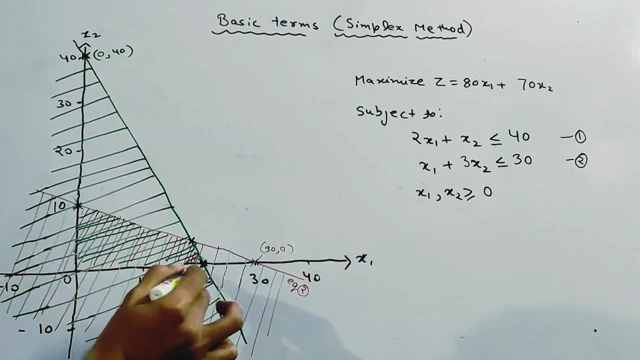 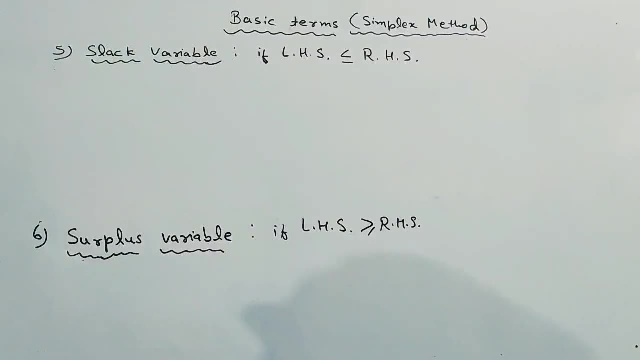 corner points of feasible region. Next is optimal solution. Optimal solution means basic, feasible solution, ki wo value jo objective function ko bhi optimize kar de. Next is slack variable: If in any constraint left hand side is less than or less than or equal to. 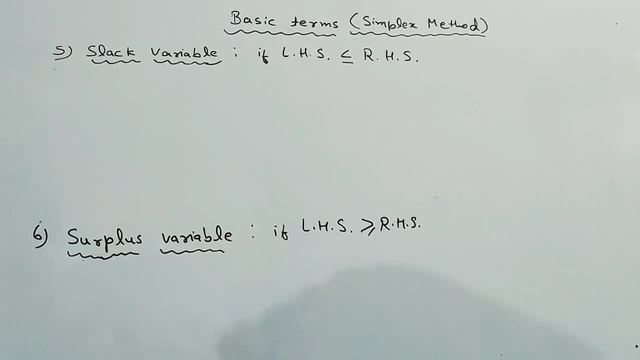 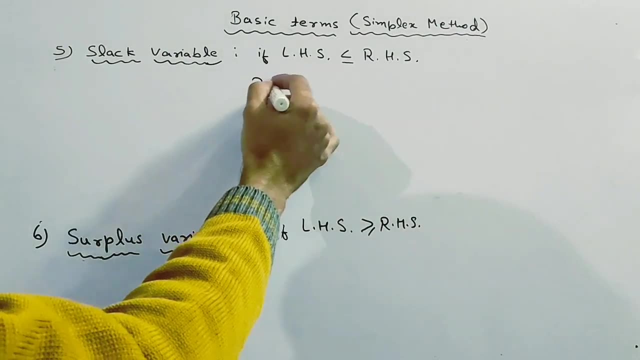 the right hand side, then to make left hand side equal to the right hand side, we will have to add something on the left hand side. For example, if 2 is less than 3, if I have to make the left hand side equal to the right hand side, then I will have to add something on the left hand side. 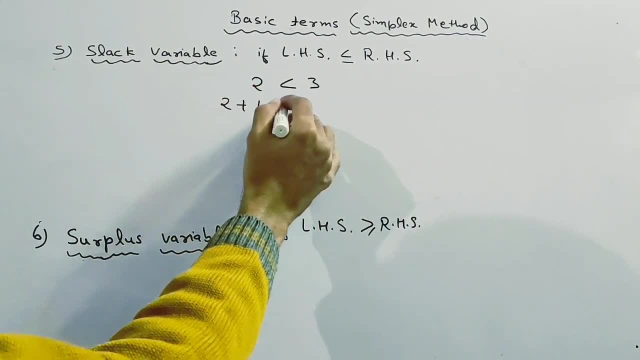 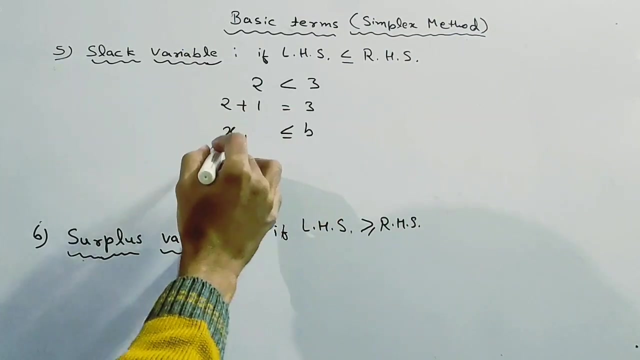 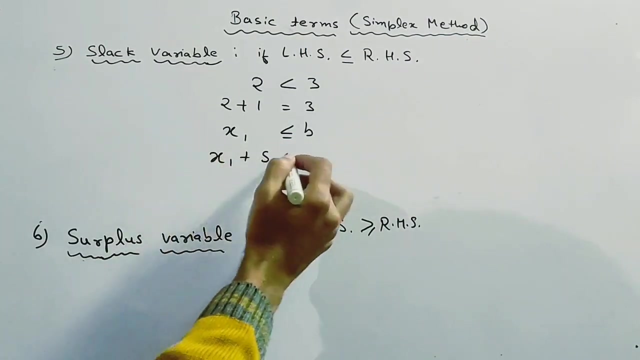 Equal to the right hand side, I will have to add 1.. So variable that we add on the left hand side to make it equal to the right hand side is known as slack variable In mathematical notation form. if x1 is less than or equal to the b, then the variable that I am denoting by s that we add on 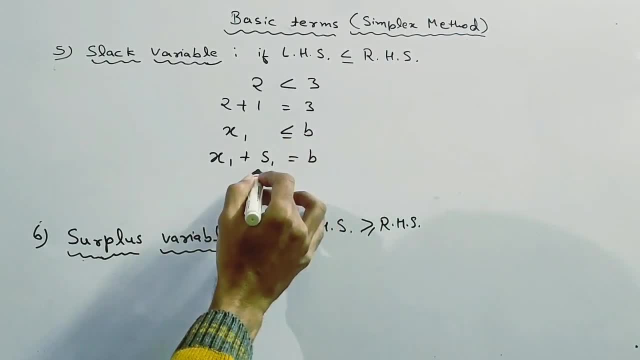 left hand side to make it equal to the right hand side is known as slack variable. Slack variable represents the unutilized resource or unutilized capacity. For example, agar kisi product ko banane ke liye machine ke 2 ghante consume hotay hain and machine humare. 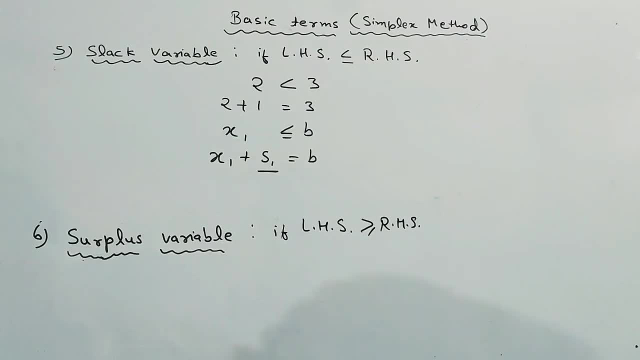 paas 10 ghante ke liye available hain to 8 ghante jo machine khali padhi raegi. these 8 hours are known as slack. Similarly, if left hand side is greater than or greater than or equal to the right, 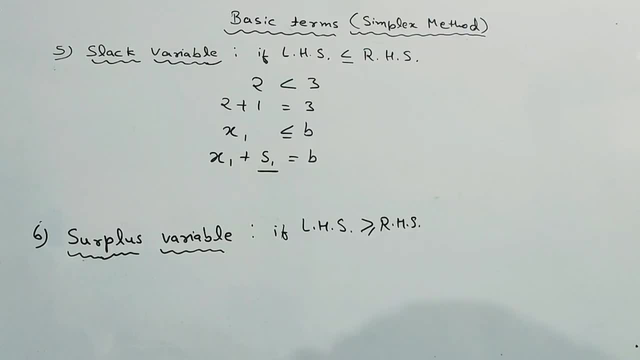 hand side, then we will have to add something on the left hand side to make it equal to the right hand side. So the variable that we subtract from the left hand side to make it equal to the right hand side is known as surplus variable. In mathematical notation form, for example, if x1 is greater than 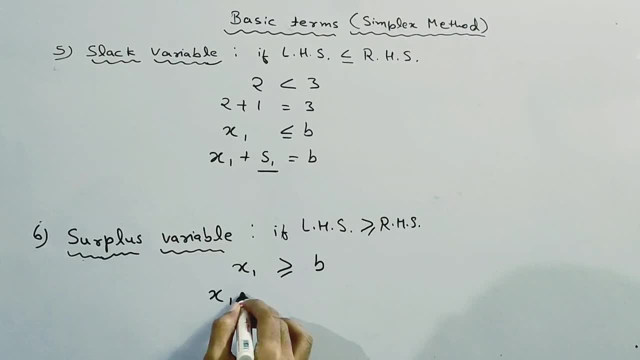 or equal to b, then the variable that I am subtracting again, I am denoting it with s in the left, so here both s are appropriate. im not calculating s, but instead im calculating the 3 dash. literally. you also do the same instead of s, from our implies. 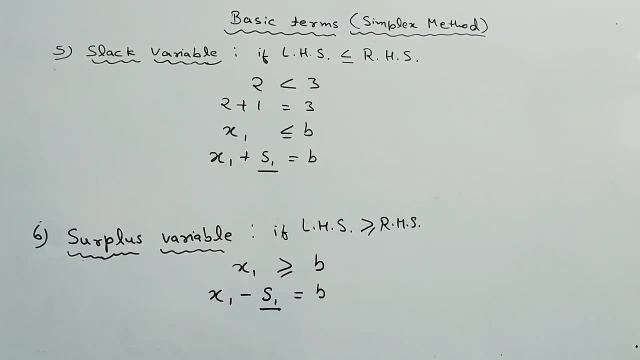 So the next variable in matrix X- ie KnowWeaknessскую what is waiting up here To make it equal to the right hand side- will be known as surplus variable. Surplus variable represents the excess amount that we have from our requirement. For exampleаз Casin ka pas, 15 kg fertilizer has been habilbale jeki field. mein 10 kg fertilizer is being used in the field. then that 5 kg extra amount is known as surplus. Next is artificial variable. if in any constraint left hand side is more than as 1 kg extra. 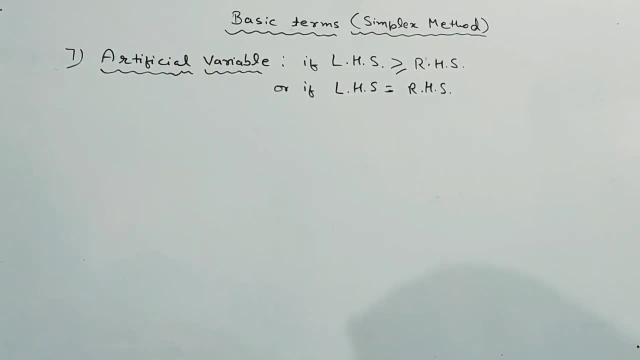 side is greater than or equal to the right hand side, or left hand side is equal to the right hand side, then we will have to add another kind of variable on the left hand side. that is known as artificial variable. There is no physical existence of artificial variable. We add this in the equation. 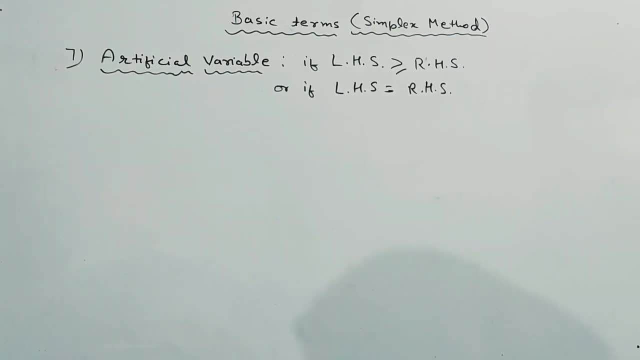 just for mathematical purpose. You can think of it as a virtual product that is not adding any value in the objective function, but it is consuming your resources and you have to get trade out of it as soon as possible. Now why do we add artificial variable in greater than or equal? 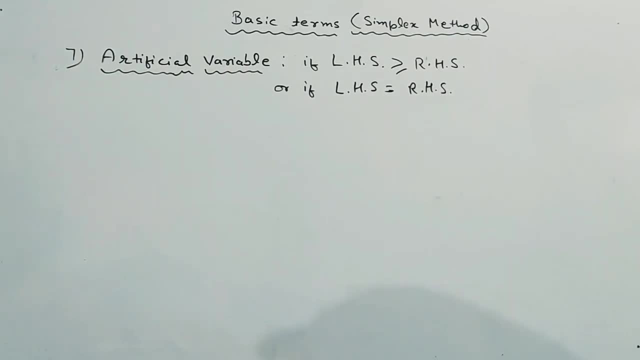 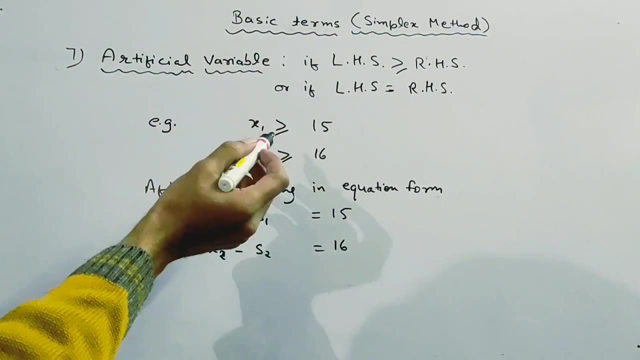 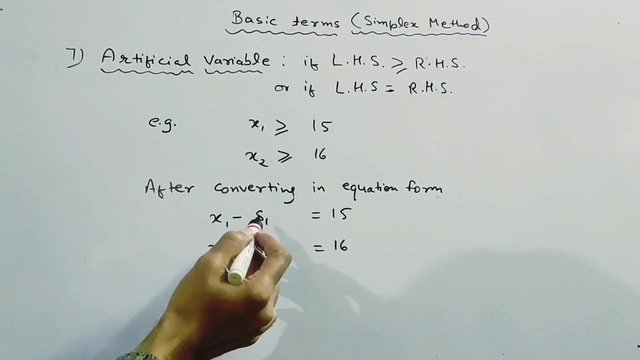 to kind of constraint or equality kind of constraint. Let's understand with some examples. For example, these are two constraints: x1 is greater than or equal to 15,. x2 is greater than or equal to 16.. To make it equal, I have subtracted the surplus variable: x1 minus s1 is equal to 15, x2 minus. 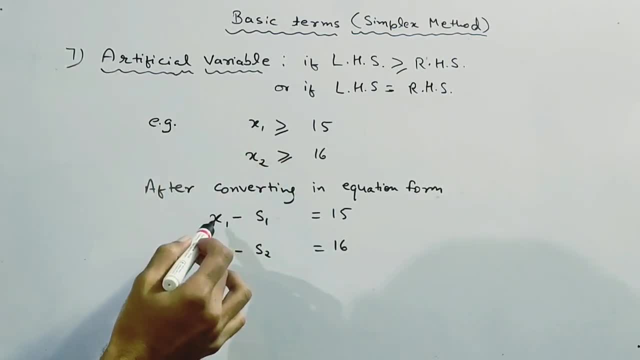 s2 is equal to 16.. Now here there are four variables: 1, 2,, 3, 4 and two equations. So we have to keep two variables zero. Suppose I keep x1 and x2 equal to zero, then my answers will be: s1, s2 is equal to minus. 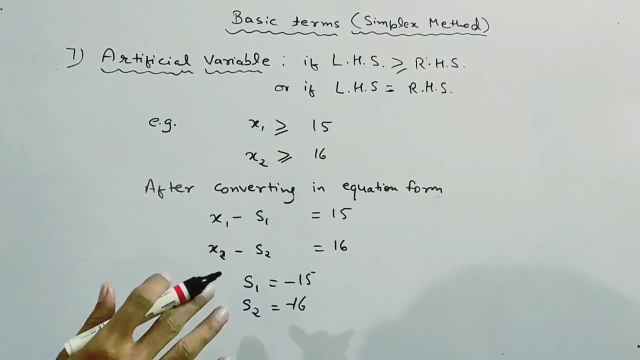 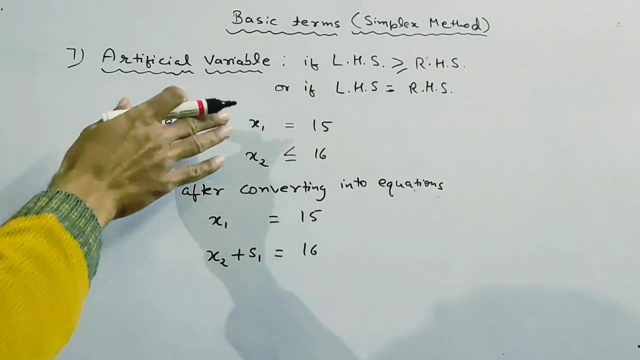 15 and minus 16.. Which is not feasible. So to negate the impact of these negative signs, we add an another variable, which is known as artificial variable. Similarly, this is the another case: X1 is equal to 15 and X2 is less than or equal to 16.. 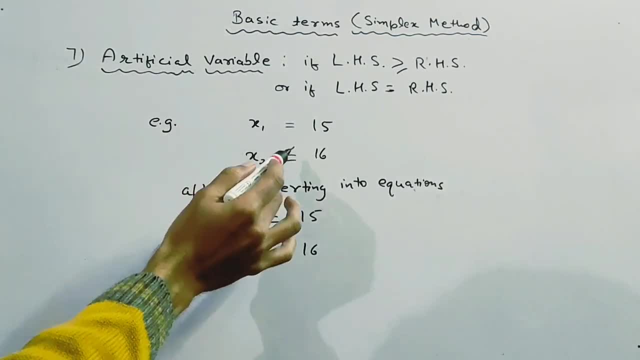 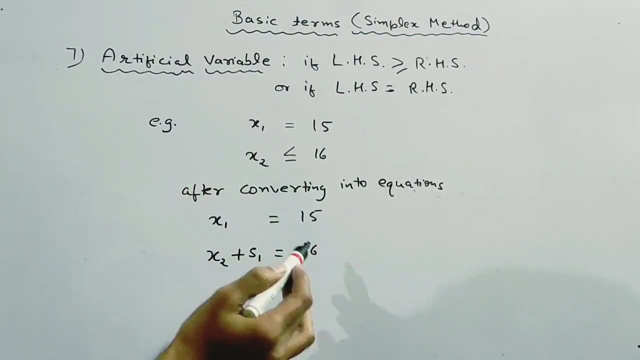 I converted this in equation form. X2 was less than or equal to 16. So I added a slack variable on the left side. That is, X2 plus S1 is equal to 16.. Now here there are 3 variables. 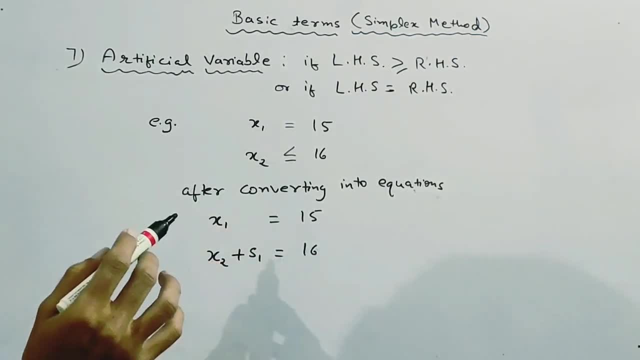 1,, 2,, 3 and 2 equations. So we have to keep 0 for any one variable. Suppose, if I keep 0 for X1,, then 0 will become equal to 15, which is not possible. 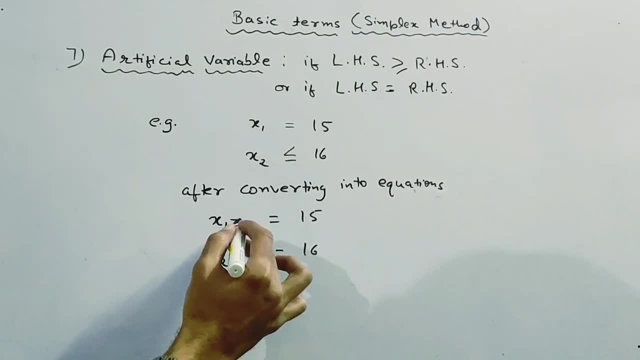 So to tackle such kind of situation, we will have to add another variable, which is known as artificial variable. So this is the other case. These are the reasons why do we add an artificial variable in the constraints: where LHS is greater than or equal to the RHS, or where LHS is equal to the RHS. 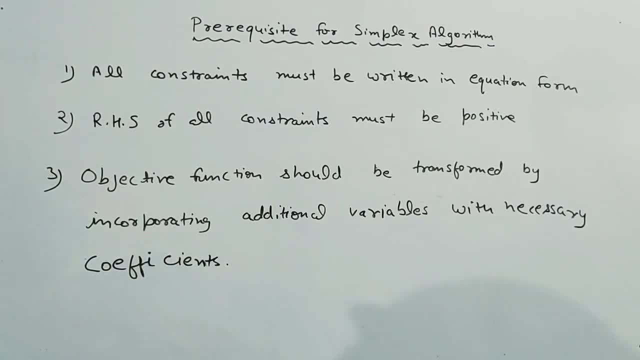 Now to solve LPP using simplex method, we have to convert all the constraints in equation form by using slack, surplus and artificial variable. Second thing, RHS of all constraints must be positive And third thing, all the additional variables which we have used to convert these equations into equation form. 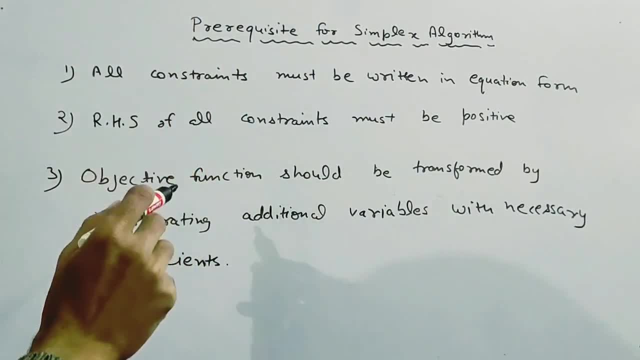 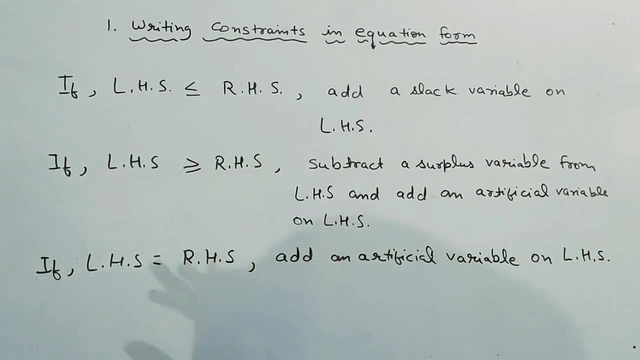 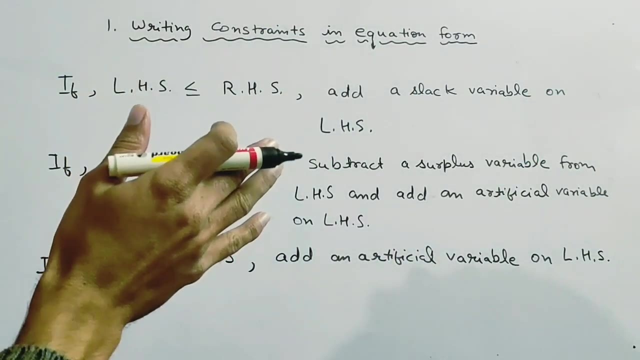 we have to add all those variables in objective function, also with necessary coefficients. Now how to convert the constraint in the equation form. If left hand side of the constraint is less than or equal to the right hand side of the constraint, then we have to add a slack variable on left hand side. 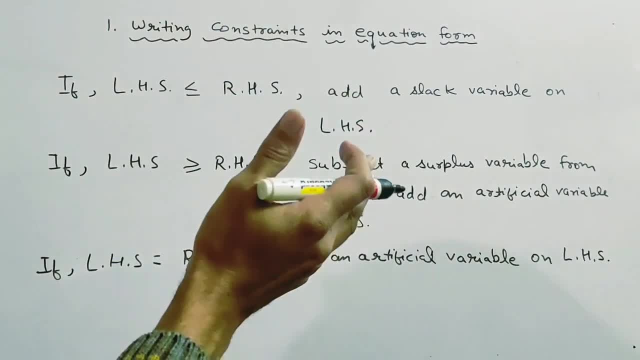 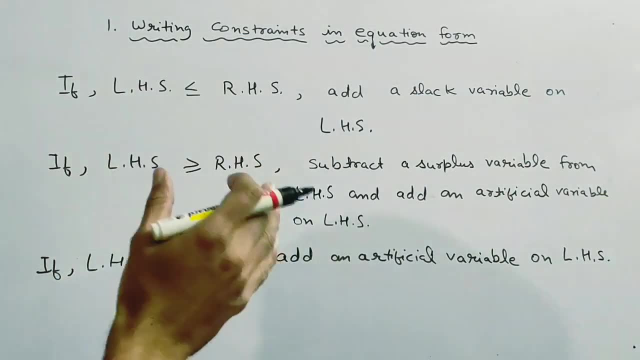 If LHS is greater than or equal to LHS, we will have to subtract a surplus and add an artificial variable on left hand side, and if LHS is equal to the RHS, we just have to add an artificial variable on left hand side. 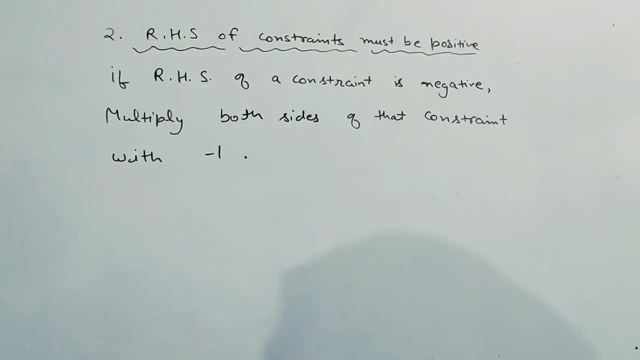 I have already told you all the reasons for all these. Now, RHS of constraints must be positive. If right hand side of the constraint is negative, then we will multiply both the sides of the constraint by minus 1.. Then we will multiply both the sides of the constraint by minus 1.. 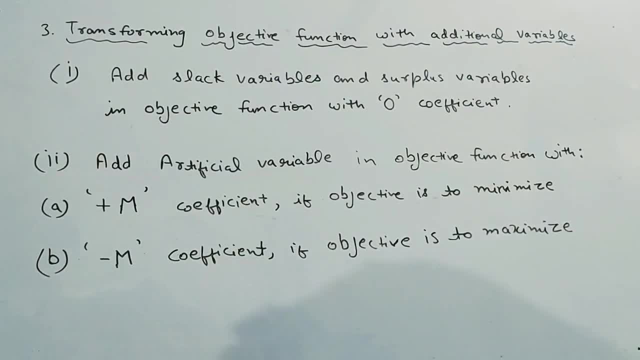 Then we will multiply both the sides of the constraint by minus 1.. Now how to transform objective function with additional variables that we have added in constraints. Add slack and surplus variables with zero coefficient in objective function, As slack and surplus variables don't add any value in the objective function. 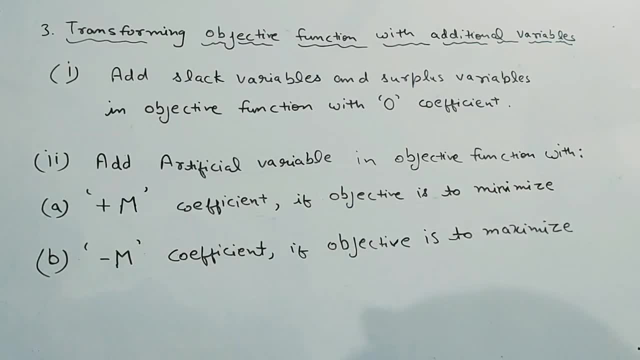 that's why we have to assign a zero coefficient to slack and surplus variable. For example, if the machine is empty for 8 hours, then it is not generating any profit for you. That's why we are assigning zero coefficient to that slack. 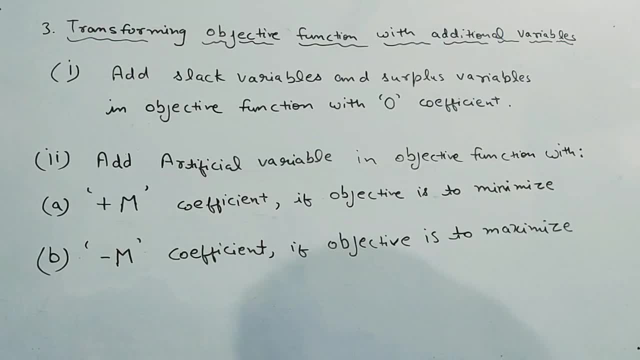 Now for artificial variable. As I earlier mentioned that there is no physical existence of artificial variable, We have added it only for mathematical purpose And we have to get rid out of it as soon as possible Because until it is in the system, we cannot optimize our objective function. 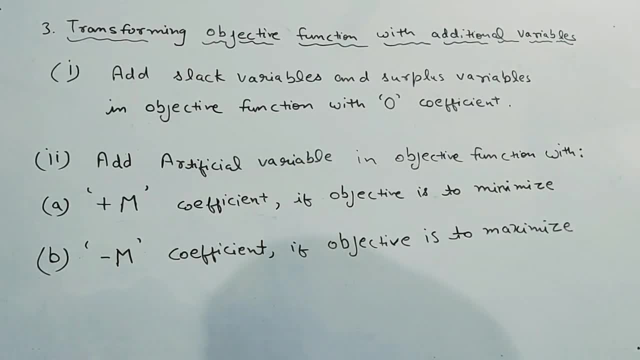 So we assign a big penalty to artificial variable in objective function. That big penalty is denoted by capital M. M is infinitely large number. If objective function is of minimization type, then we add artificial variable with positive m coefficient in objective function. 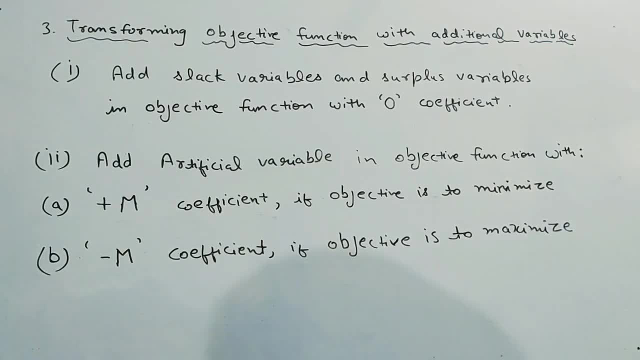 And if objective function is of maximization type, then we add artificial variable with minus m coefficient, Because until artificial variable with positive m coefficient exists in minimization type of objective, we cannot minimize our objective function. Similarly, in case of maximization type of objective, 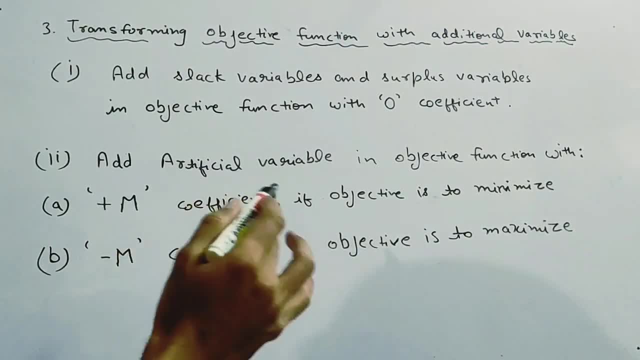 until negative m, a exists, we cannot maximize our objective function. Always, the value which will come in objective function will be approximately of negative infinity. Artificial variable is like a cancer that is consuming our resources but not adding any value in the system. Let's take some examples. 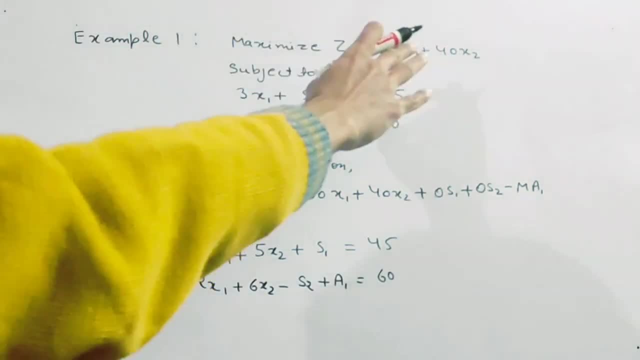 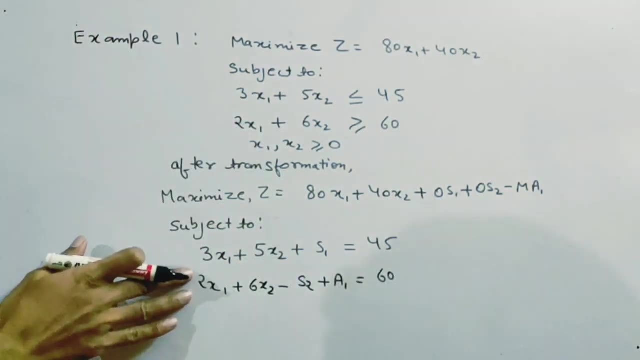 First example is: maximize z is equal to 80x1 plus 40x2. subject to this, First of all we have to write these constraints in equation form: Less than or equal to type of constraint. So on the left hand side we will add slack variable. 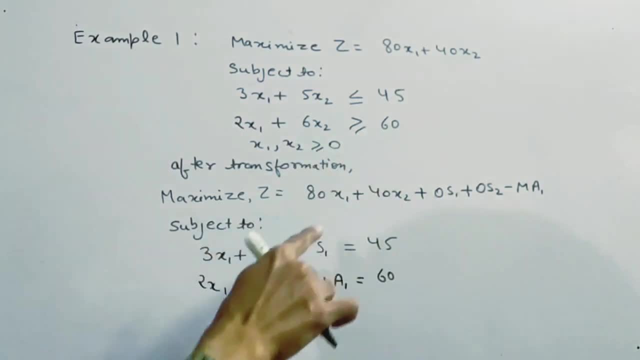 Greater than or equal to type of constraint. So on the left hand side we subtract a surplus variable and add an artificial variable, Now the new additional variable which we have added. we have to add them in objective function also. So slack and surplus variables are added with zero coefficients. 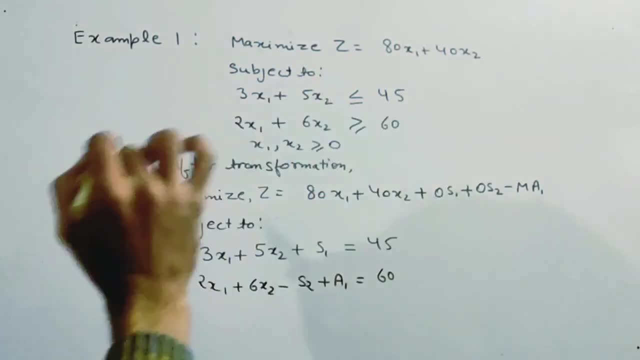 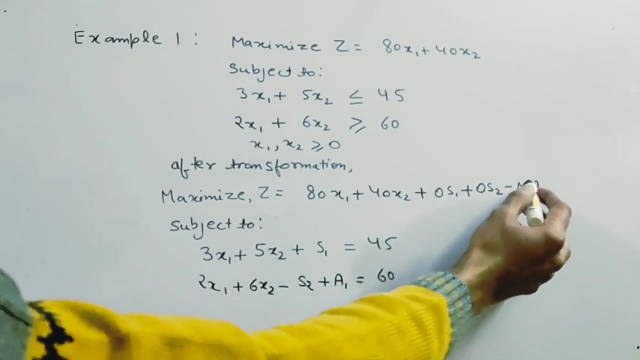 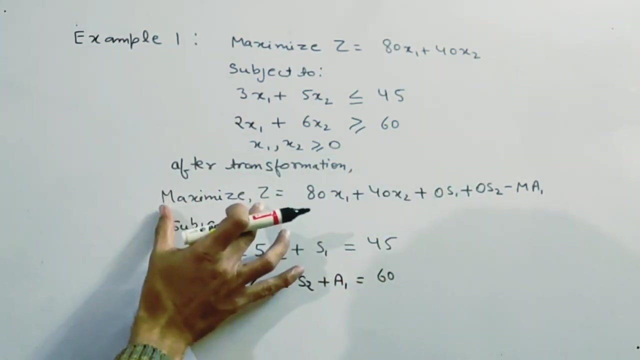 as they don't add any value in the objective function, While artificial variable is added with a big negative m penalty, Because till the time this negative m is in this system, we cannot maximize it. Whatever value of x1, x2, s1, s2 comes, 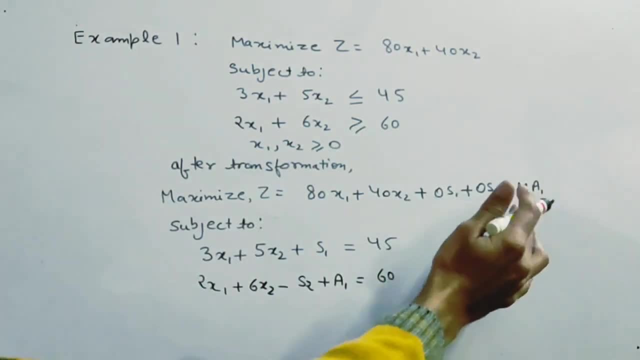 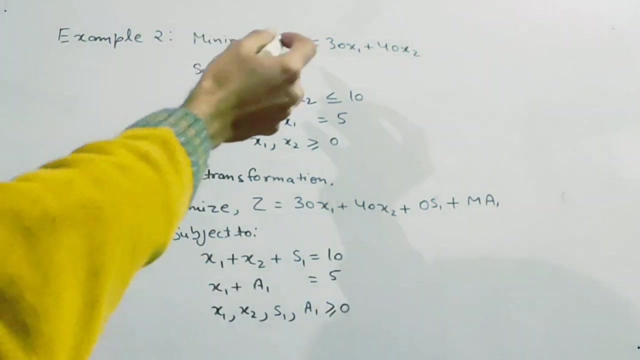 but overall the value of objective function will be approximately of negative m or negative infinity, So we have to get rid out of it as soon as possible. Let's take another example, that is, minimize z is equal to 30x1 plus 40x2. subject to these constraints, 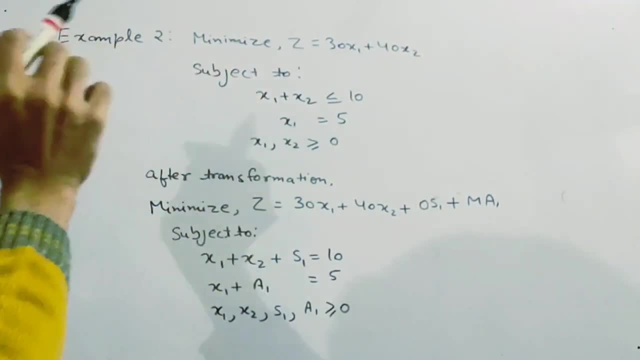 First of all, we have to write these constraints in equation form: Less than or equal to type of constraint. So I added a slack variable on the left hand side, And next is equality- type of constraint. So here I have added only one artificial variable. 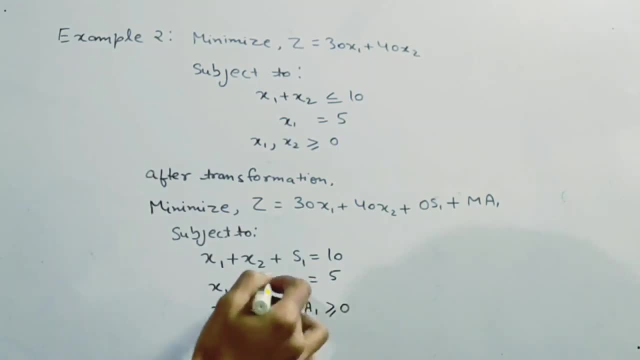 Now we have to add these new variables in objective function also. So slack variable has been added with zero coefficient, Whereas artificial variable, because it is a case of minimize Artificial variable- has been added with a big positive m penalty, That is plus m a1.. 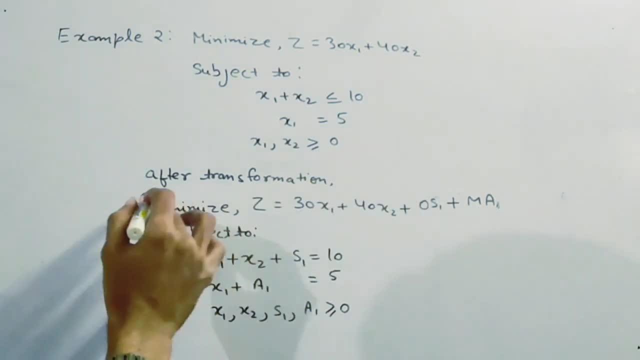 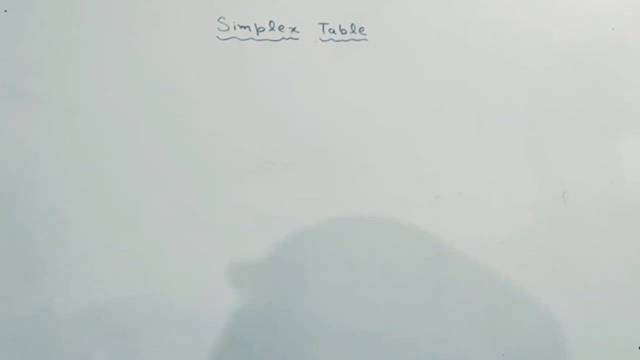 Till the time this is in the system, we cannot minimize this objective function, And x1,, x2, s1, a1 must be greater than or equal to zero. After transforming all constraints and objective function, we have to write all equations in a tabular form for calculation purpose. 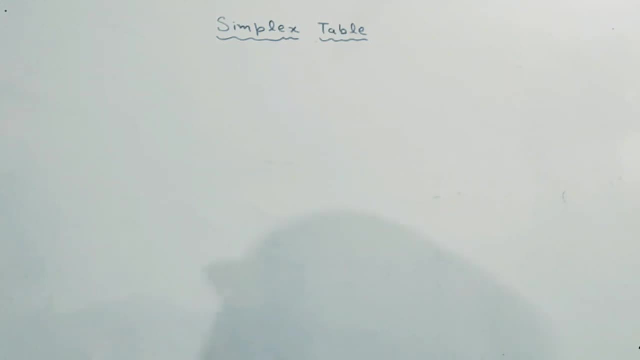 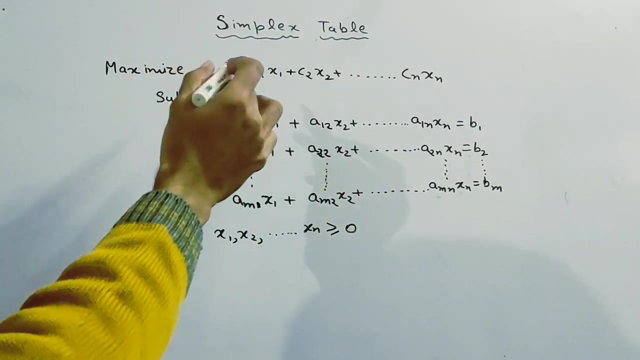 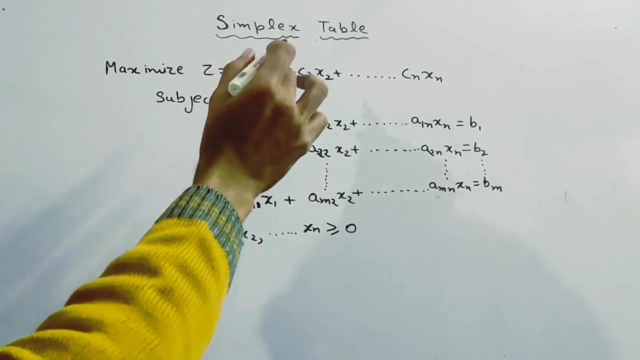 That table is known as simplex table or simplex tableu. Suppose after transformation we get to see some such equations. There are n number of variables in objective function, including slack, surplus and artificial variables. I have not represented any variable with s or a. 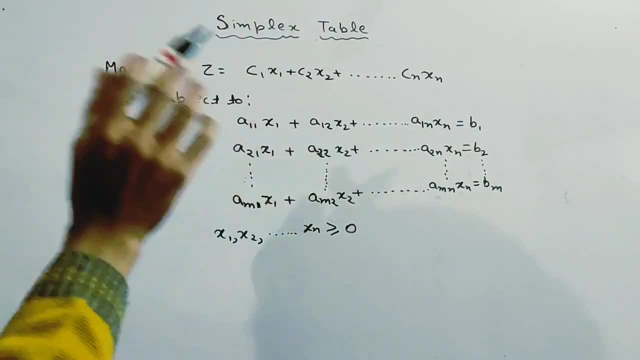 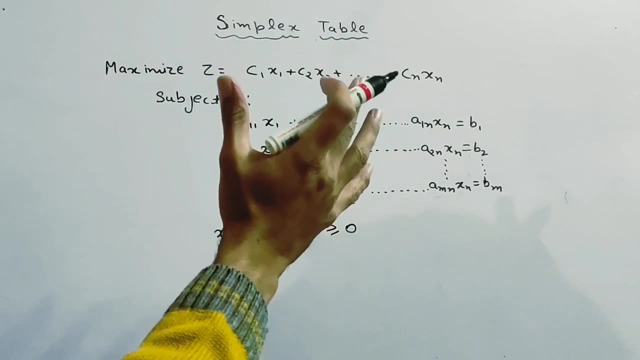 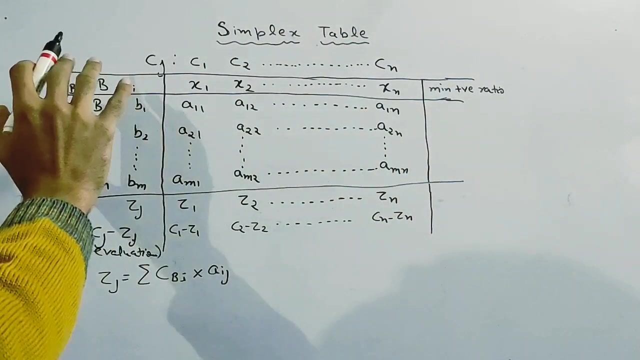 And there are m number of equations. So for calculation purpose we have to write the data of all these equations in a tabular form. That table is known as simplex table. Structure of simplex table looks something like this: This part is known as basis and this part is known as body matrix. 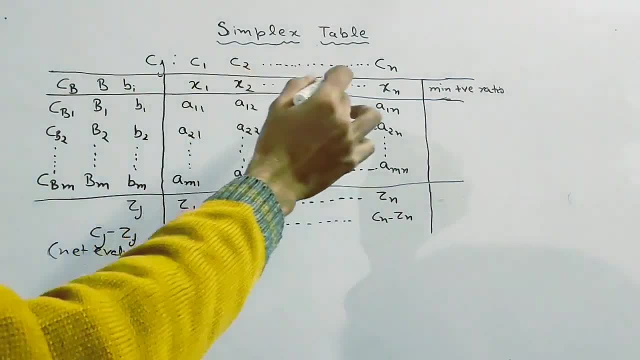 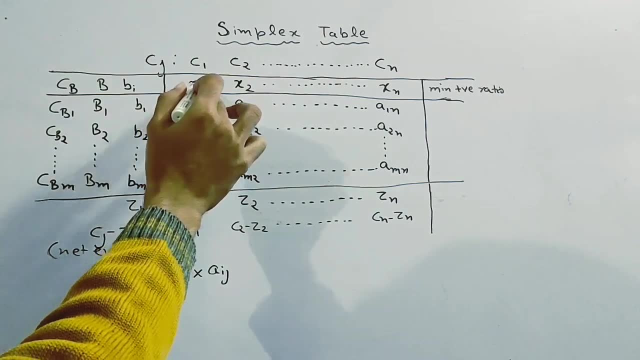 First of all, in objective function, all the variables, including slack surplus and artificial variables. we write them here. For example, in this case I have noted down x1, x2, up to x1 here On top of this. 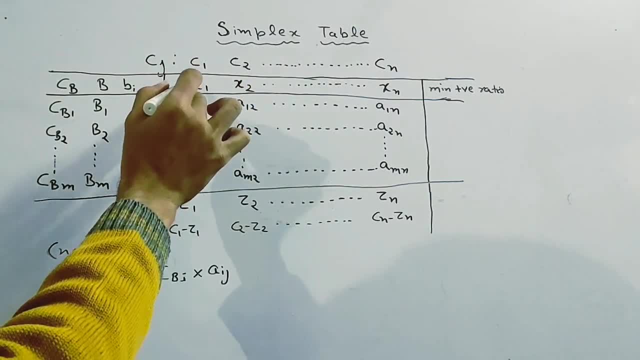 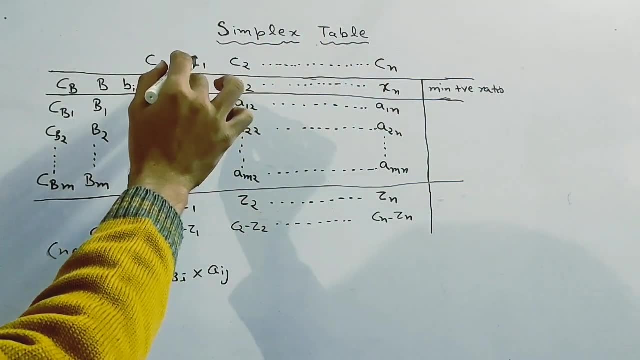 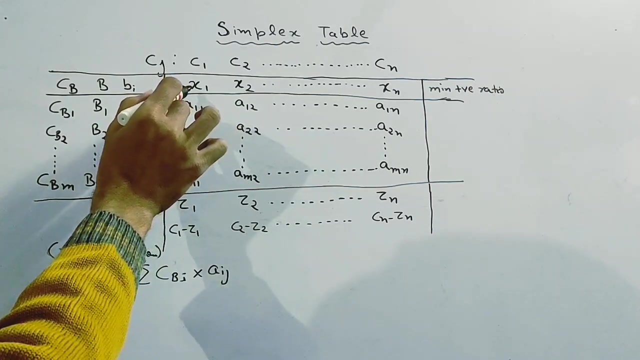 we note down all the coefficients of these variables in objective function, For example c1, c2 up to cn. Coefficient represents the contribution that variable is making in our objective function. For example, one unit of x1 is contributing c1 unit in objective function. 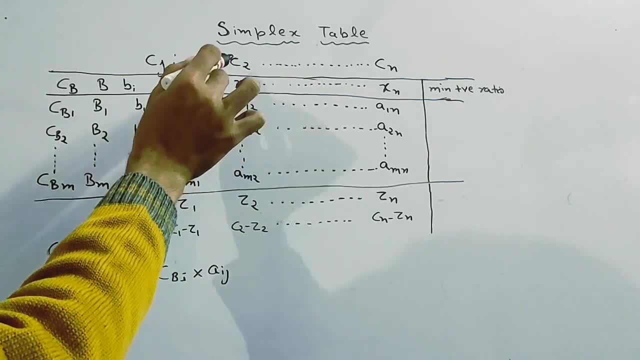 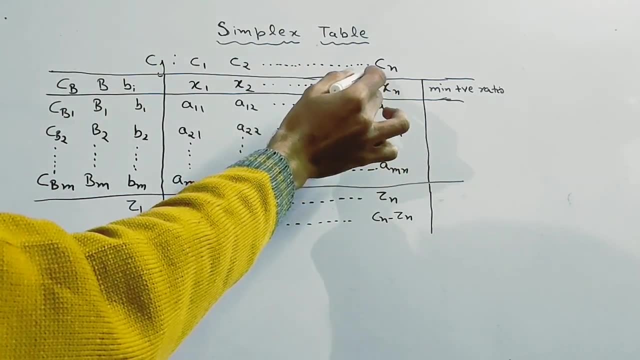 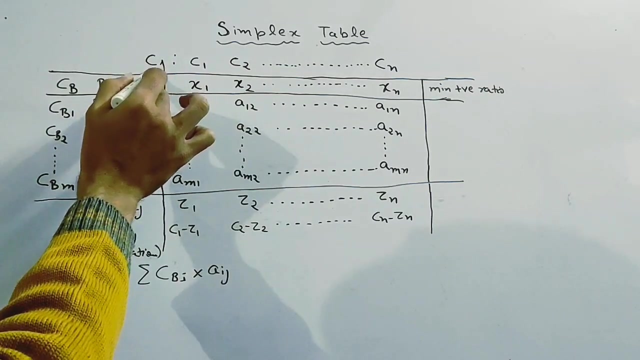 Similarly, one unit of x2 is contributing c2 units in objective function. Similarly, one unit of xn is contributing cn units in objective function. We represent these coefficient values by cj. j means column number. For example, if it is the first column, it is c1.. 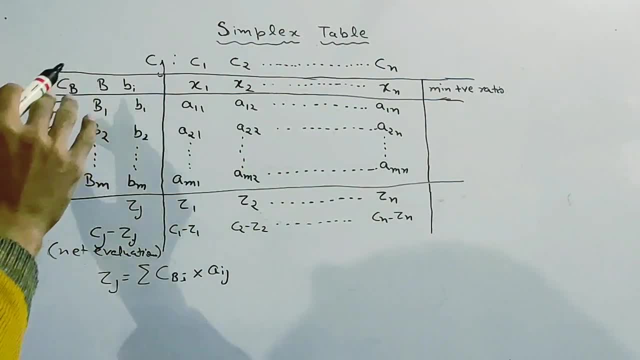 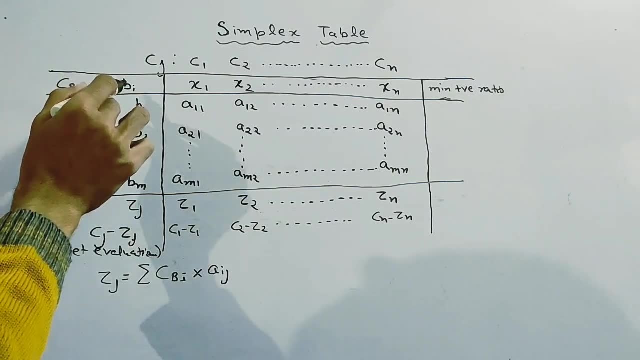 If it is the second column, it is c2 and so on. In basis we show basic variables, coefficient of that basic variables in objective function And solution value of that basic variable. For example, here there are m equations and n variables. 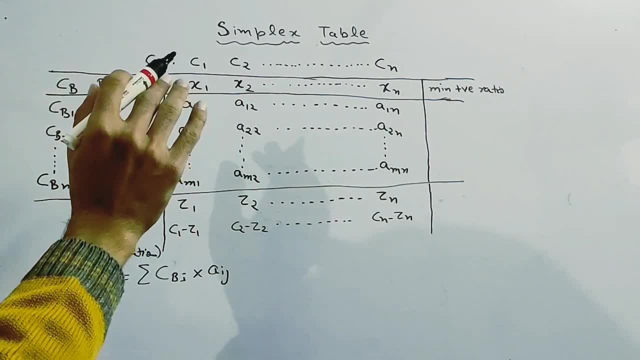 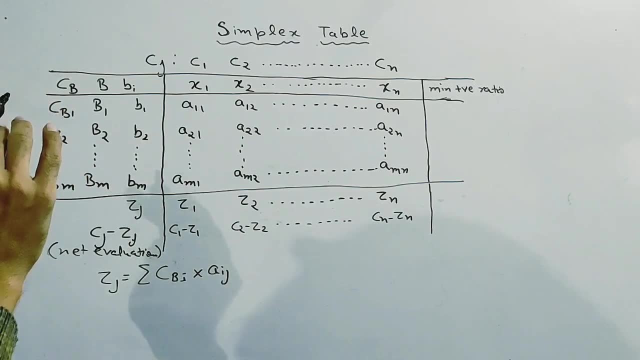 So we have to keep n minus m variable as 0. These n minus m variable will be known as non-basic variable And the remaining variables that are left, that is m variables, that will be known as basic variable. We note down those basic variables below capital B. 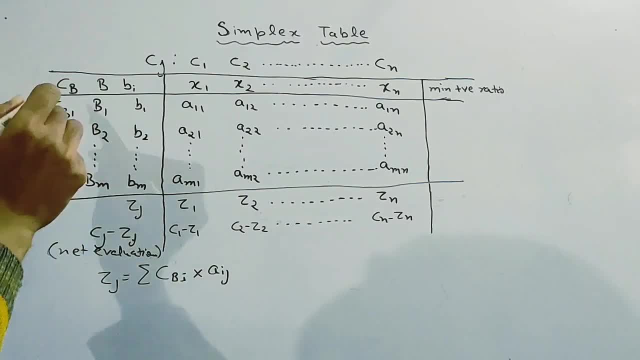 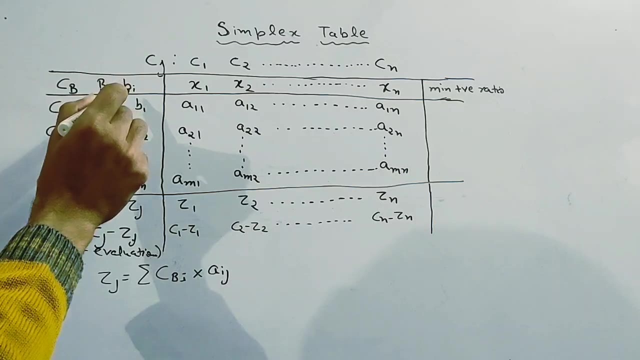 That is b1, b2 up to bm. Below cb we note down their coefficient in objective function And below bi we represent their solution value. i means row number. For example, for first row it is b1.. For second row it is b2.. 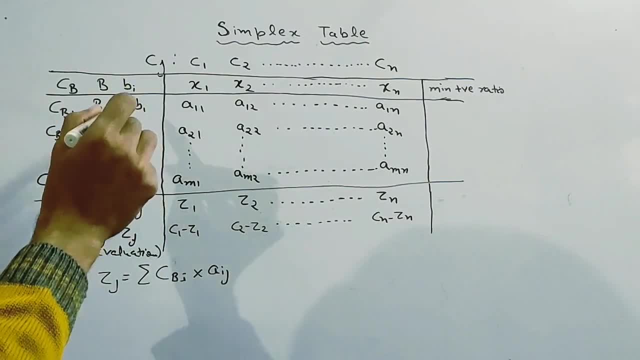 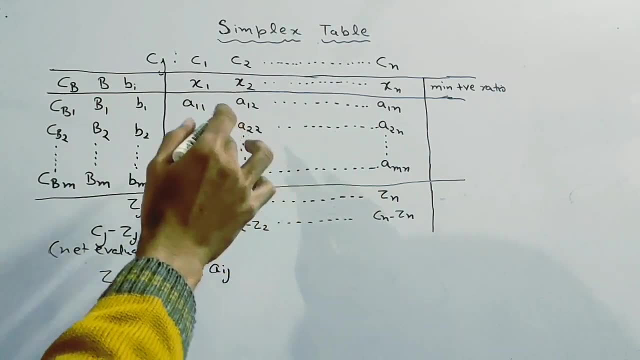 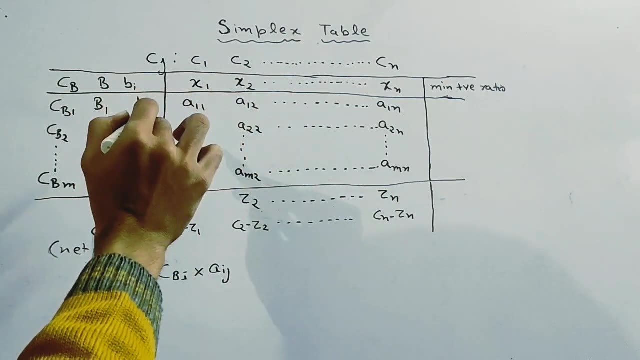 And for mth row it is bm. There are m variables, so there will be m rows. In body matrix we show aij values. aij values are the coefficient of these variables. in equation ij represents i number's row and j number's column. 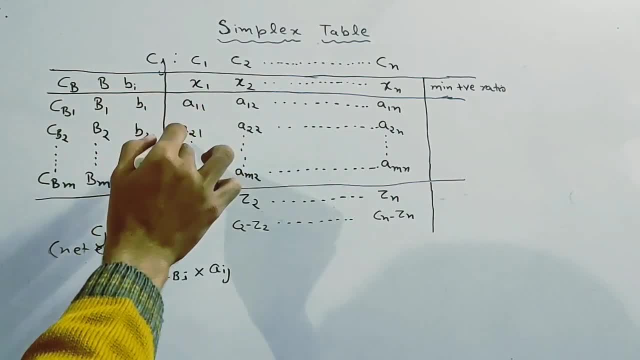 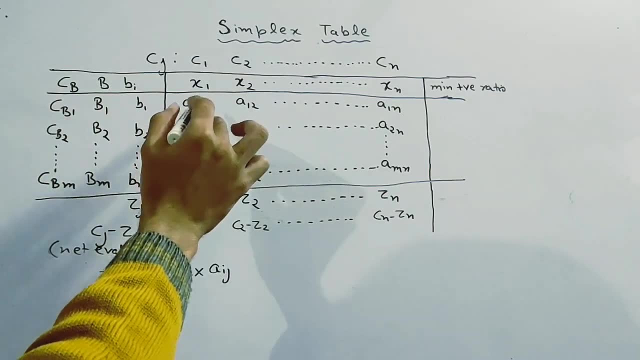 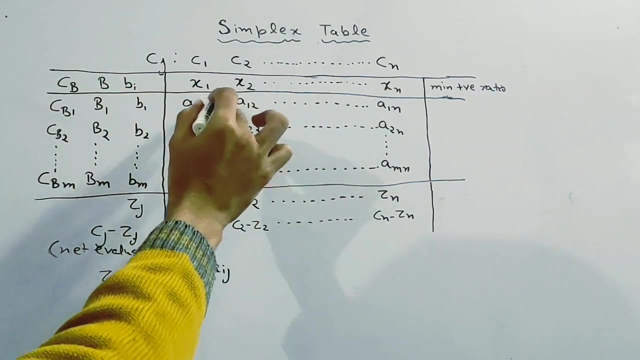 For example, a11 is first row, first column, a21 is second row, first column And ij also represents the coefficient of jth number's variable in i number's equation. For example, in first equation we have written all the coefficients of these variables here. 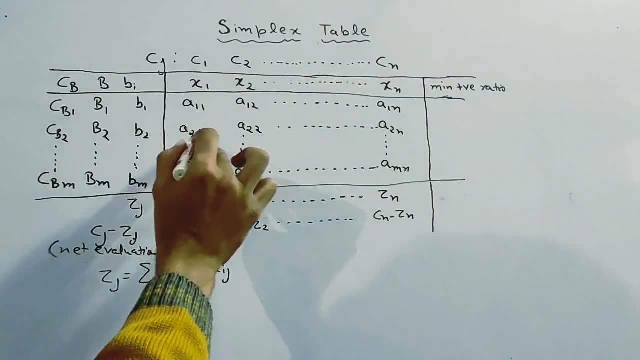 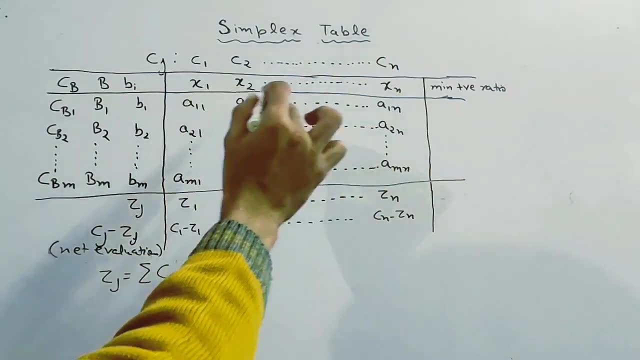 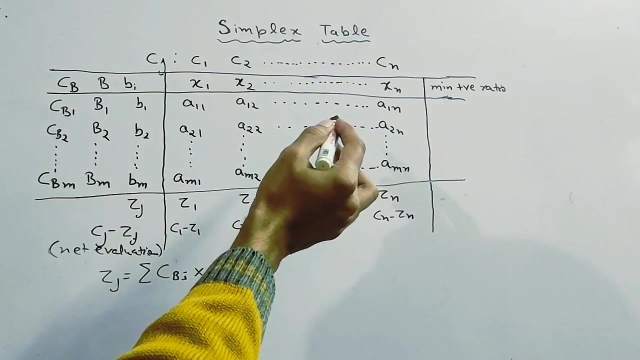 In second equation. we have written all the coefficients of these variables here And there are m- number of equations and n- number of variables. So there are m into n aij values. We get aij values directly from equations. m is from equations and m is from rows. 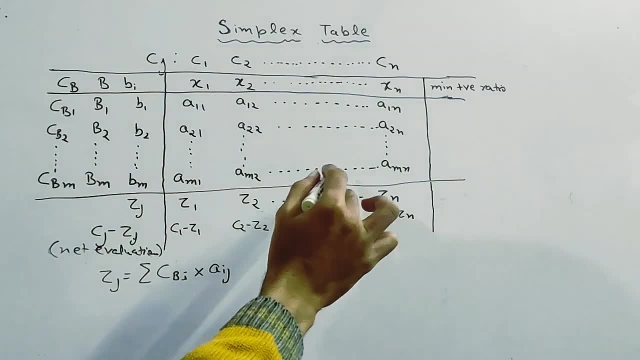 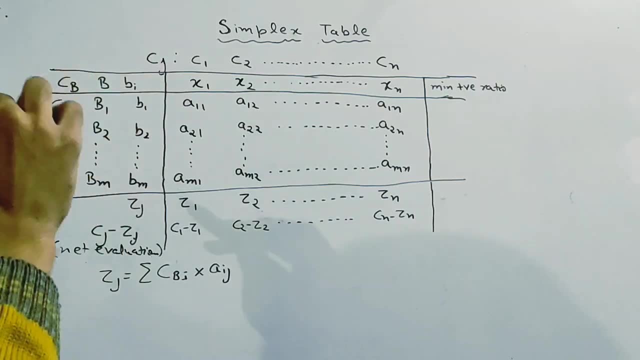 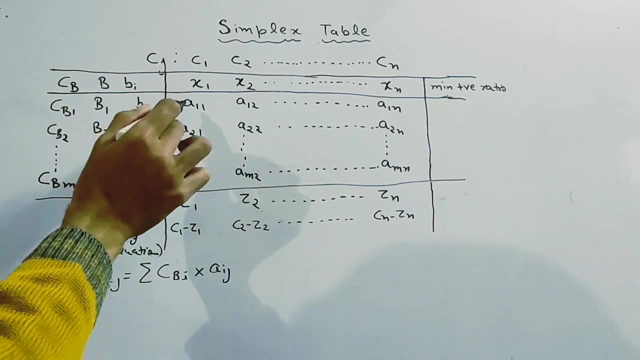 As it is. we note down these coefficients from equations. aij value represents the marginal rate of substitution between variables. For example, if we want to produce one unit of x1,, then we have to sacrifice a11 units of b1.. Similarly, if we want to produce one unit of x2,. 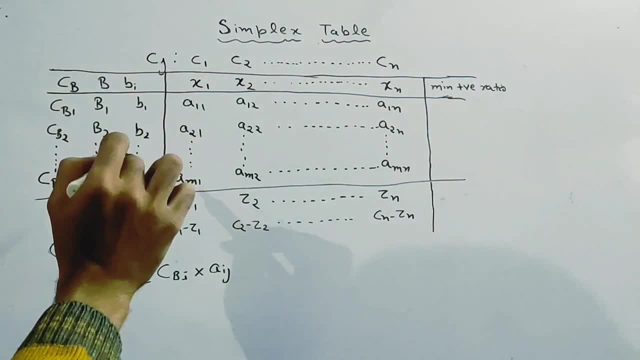 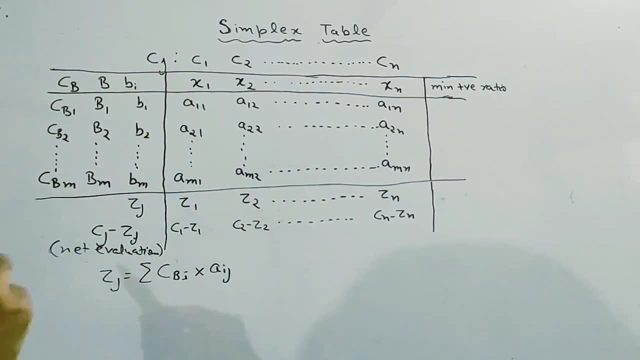 then we have to sacrifice a22 units of b2.. Now we have to see whether this solution is optimal or not. For that we need to calculate zj values. zj represents the outgoing profit or reduction in the objective function value if jth variable is introduced in the system. 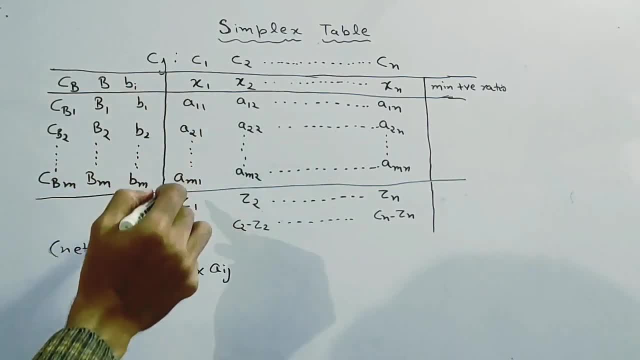 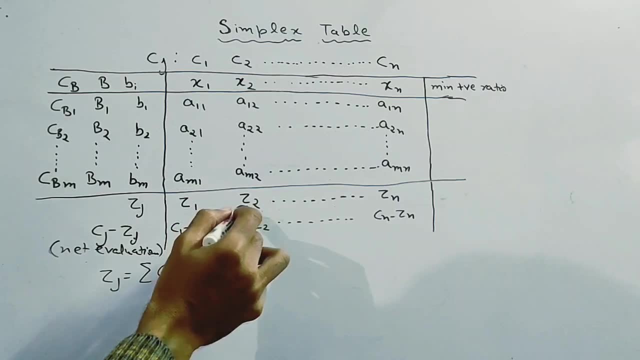 For example, if we produce one unit of x1,, then we will have a loss of z1 unit. Similarly, if we produce one unit of x2, then in objective function we will have a reduction of z2 value. zj values are calculated by this formula. 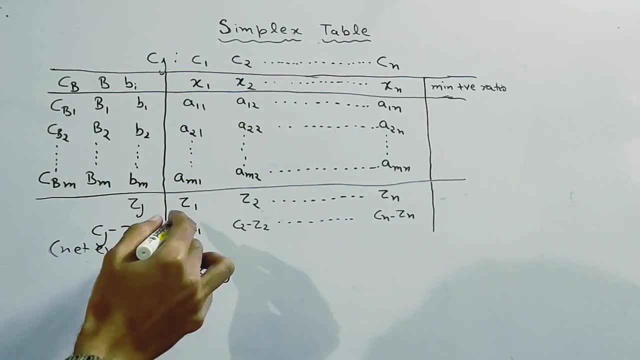 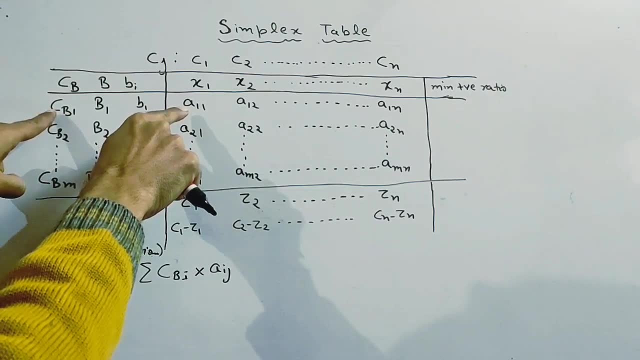 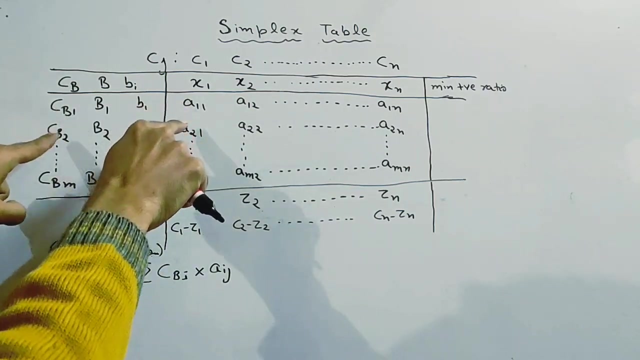 For example, the column of which you have to calculate zj values, multiply the aij values of that column by the corresponding cb value and add them, For example, for calculating z1,, this into this plus, this into this plus, and so on. 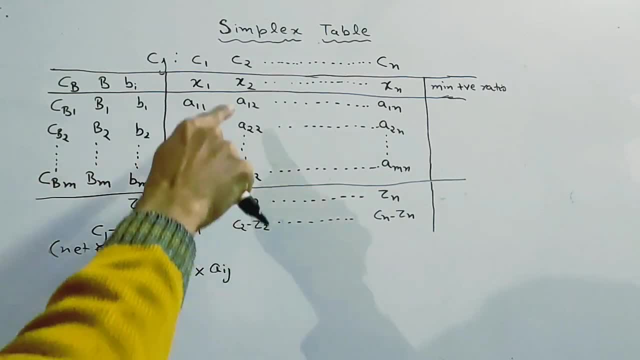 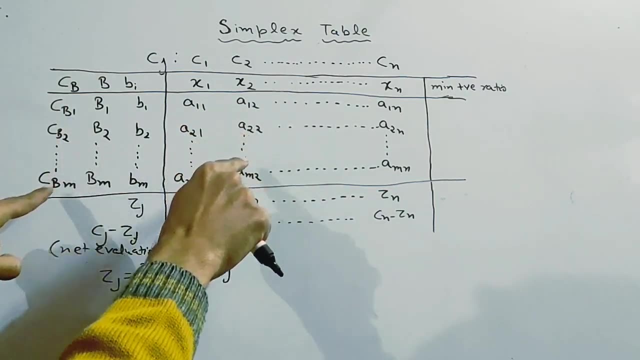 up to this into this. Similarly for calculating z value of second column, cb1 into a12, plus cb2 into a22, up to cbm into am2 and so on. Next we have to calculate cj minus zj values. cj minus zj value row is also known as: 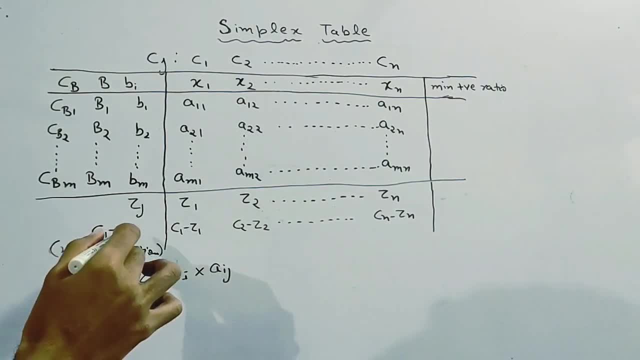 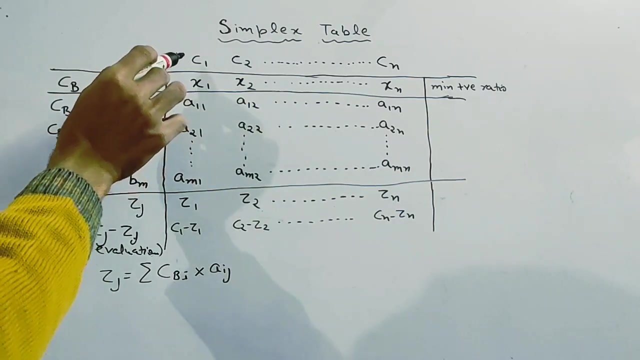 net evaluation row or index row. cj minus zj value represents the net change in the objective function by introducing a variable. For example, cj values are representing the contribution that a variable is making in objective function, While z1 is representing the outgoing contribution. 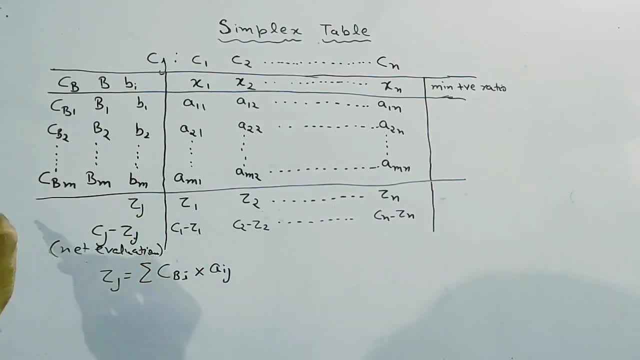 if variable is introduced in the system. For example, if we produce one unit of x1, then c1 unit will be added in objective function But we will have a loss of z1.. So what will be the net change? That is c1 minus z1.. 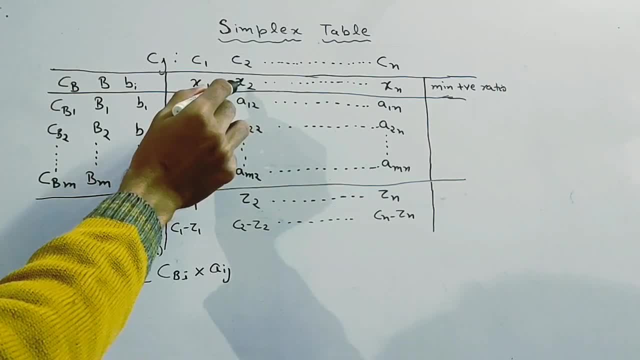 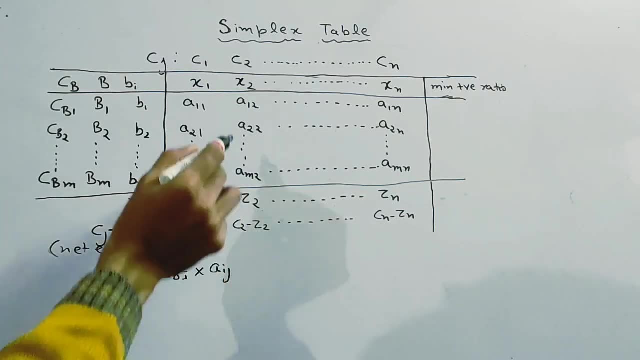 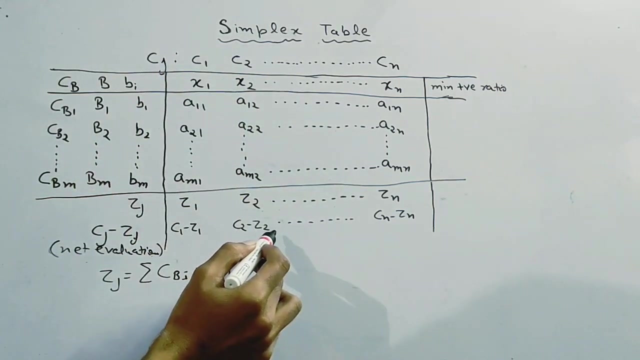 Similarly, if we produce one unit of x2, then addition of c2 units will be there, but exit of z2 units will be there. So what will be the net change? By introducing one unit of x2 variable will be given by c2 minus z2.. 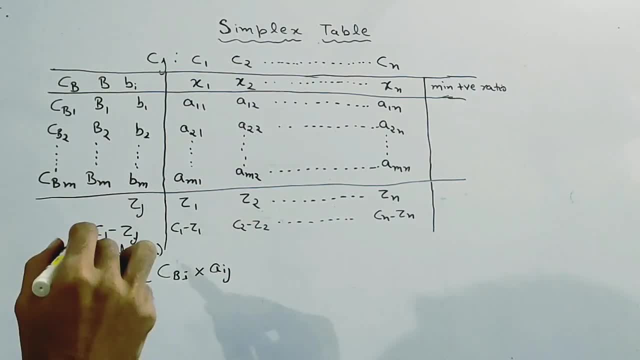 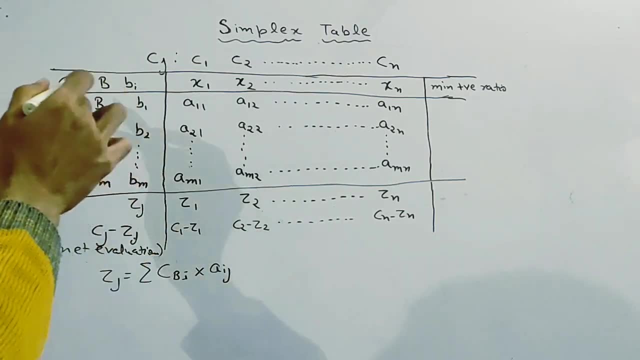 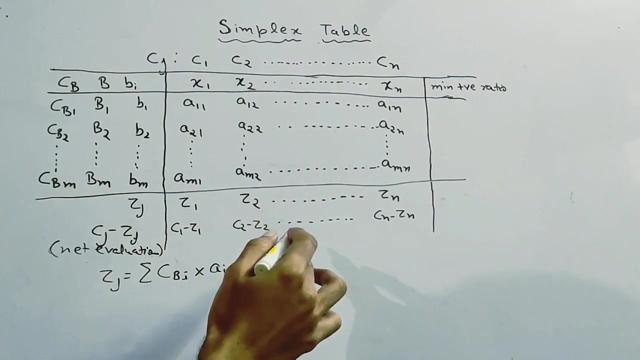 If in a maximization type of objective function all cj minus zj values are 0 or negative, then our solution is optimal Because there is no scope of improvement. All cj minus zj values are either 0 or negative. Similarly, 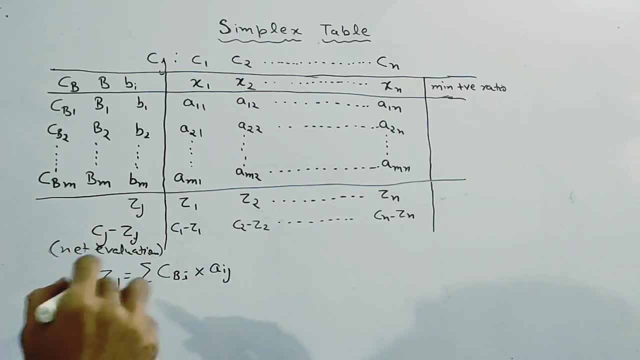 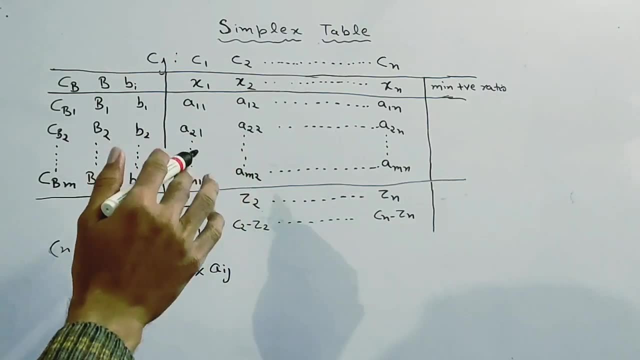 in case of minimization type of objective, if all cj minus zj values are 0 or positive, then there is no scope for further improvement. The solution is optimal. But if this is not the case, then we will move on to our next step. 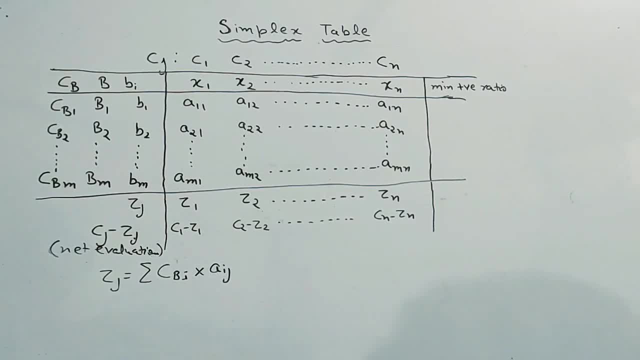 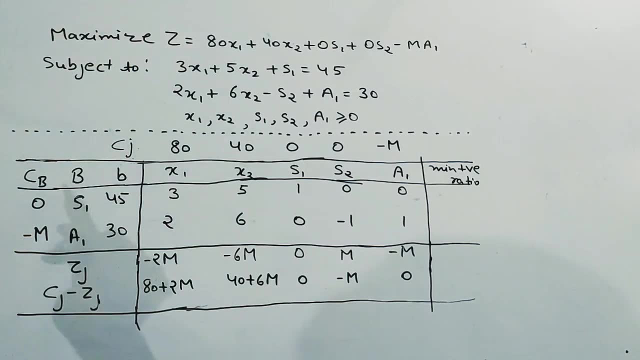 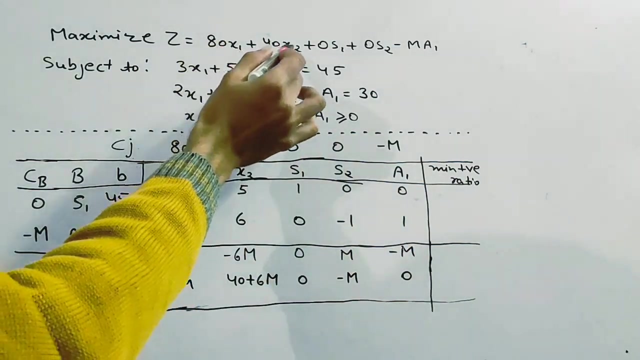 which we will discuss in the next part. Let's take an example from our earlier discussion. These are the equations after transformation In the simplex table. first of all, we have noted down all the variables in the objective function, That is, x1, x2, s1, s2 and a1. 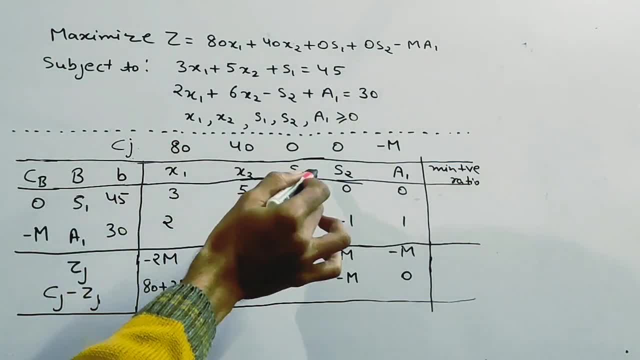 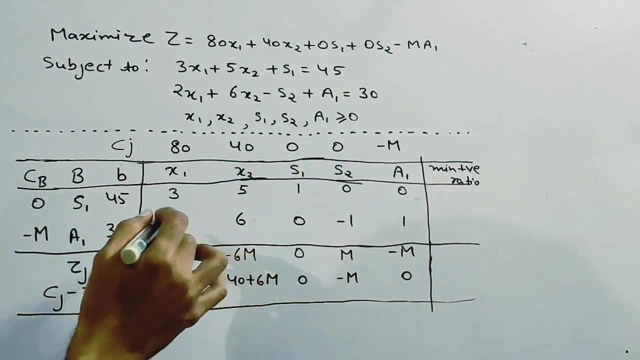 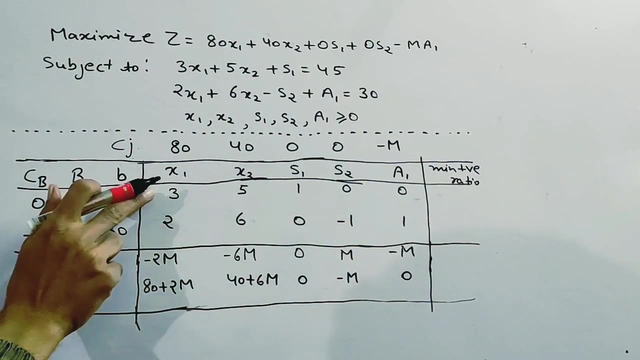 On top of that we have noted down all the coefficients in the objective function, That is 80,, 40,, 00 and minus m In the body matrix. we have noted down all the coefficients for all these variables. For the first equation we have noted down the first row. 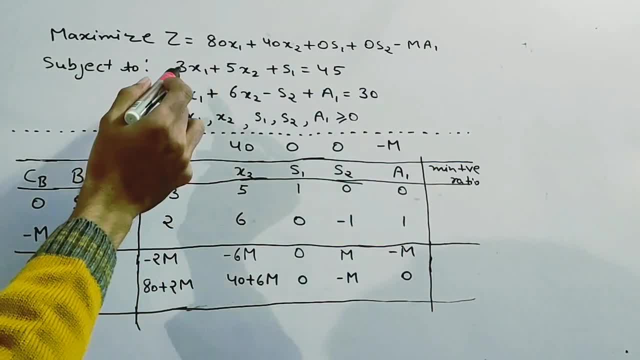 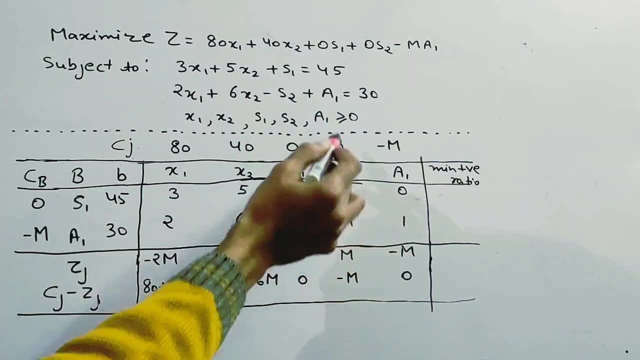 And for the second equation, we have noted down the second row. For example, in the first equation, x1 has a coefficient of 3, x2 has a coefficient of 5, s1 has a coefficient of 1, s2 is not there. 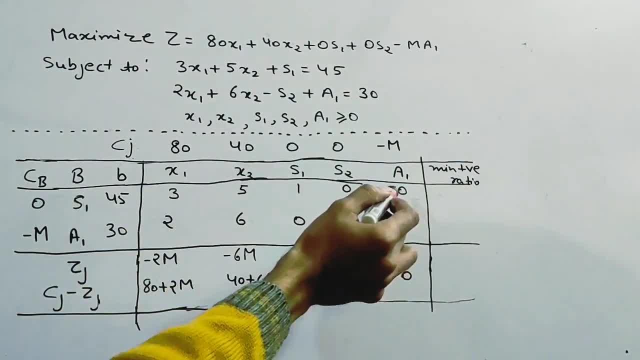 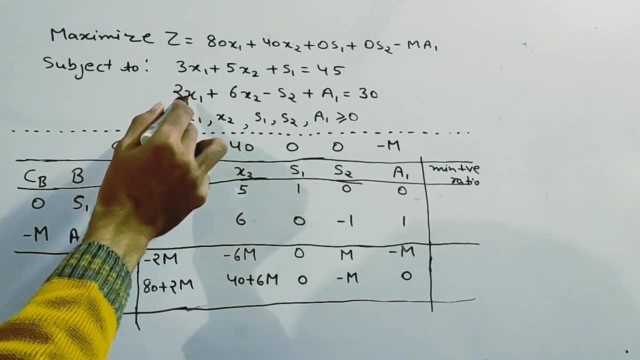 that's why it is a 0 coefficient. a1 also is not there, so it is a 0 coefficient. Then, in the second row, we will note down all the coefficients from the second equation. x1 has a coefficient of 2,. 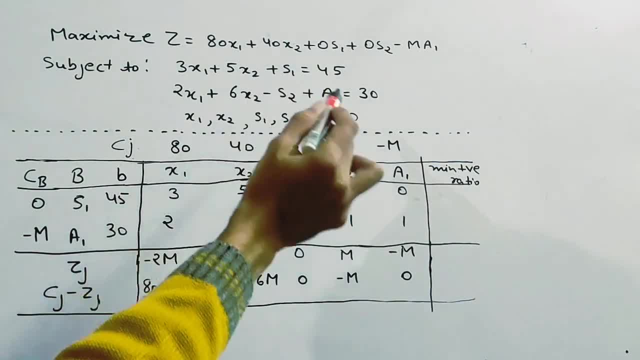 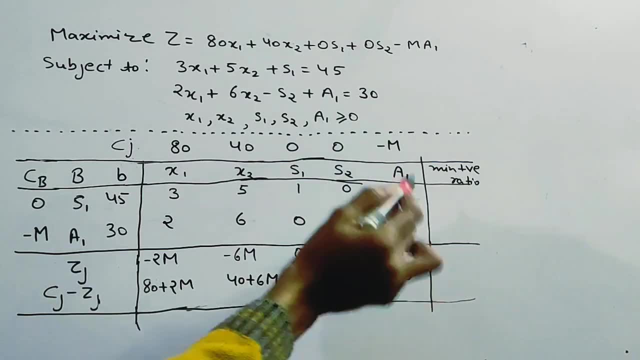 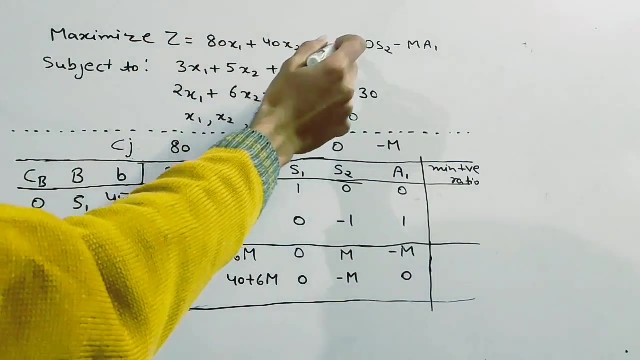 x2 has a coefficient of 6, X2 is 6, S2 is minus 1, S1 is not there, so 0 coefficient. A1's coefficient is 1, which we have not downed here. Let's talk about our basic solution here. there are 5 variables: 1, 2, 3, 4, 5 variables. 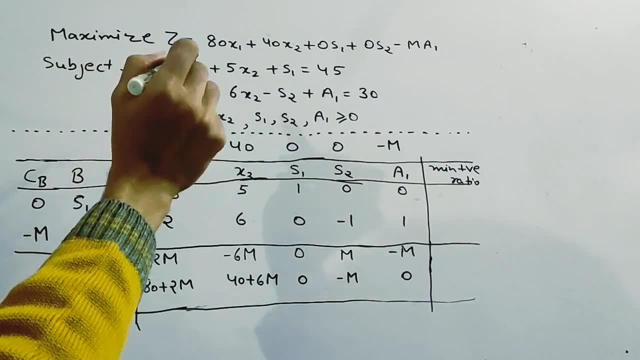 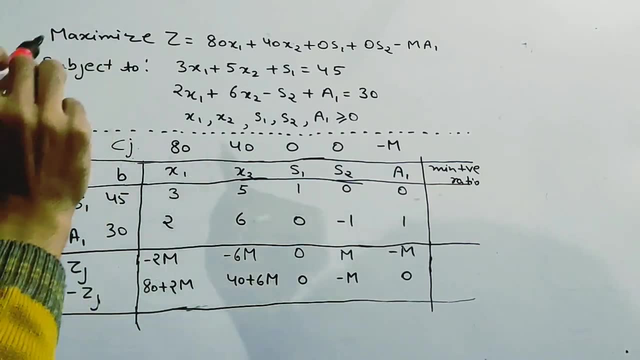 are there, whereas there are 2 equations. so 5 minus 2, that is 3, we have to keep 3 variables as 0.. The variables which we will keep as 0, they will be our non-basic variables and those: 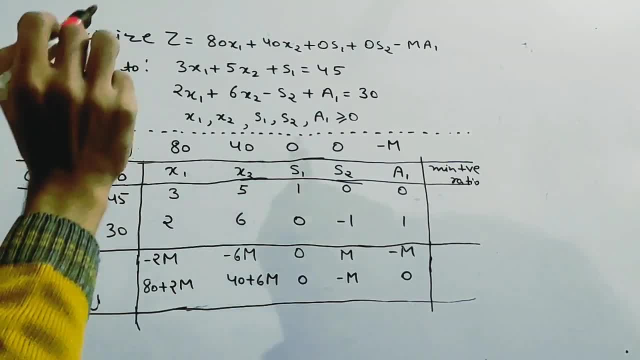 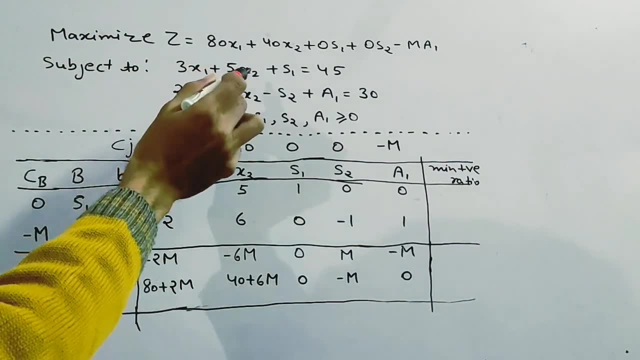 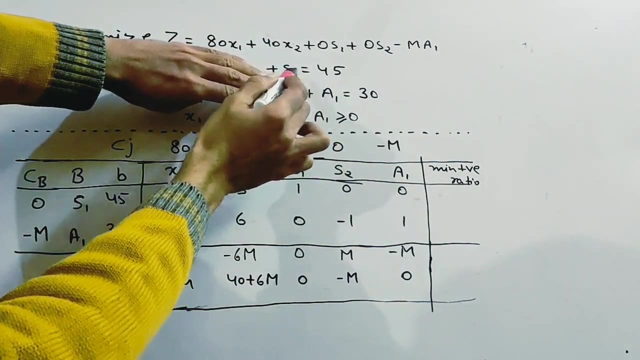 which will be left will be our basic variables. So, first of all, we always keep decision variables and surplus variables as 0,. so 1,, 2, 3, we kept these 3 variables as 0.. We have S1 and A1, these 2 are our basic variables. we have noted them down below capital B: S1. 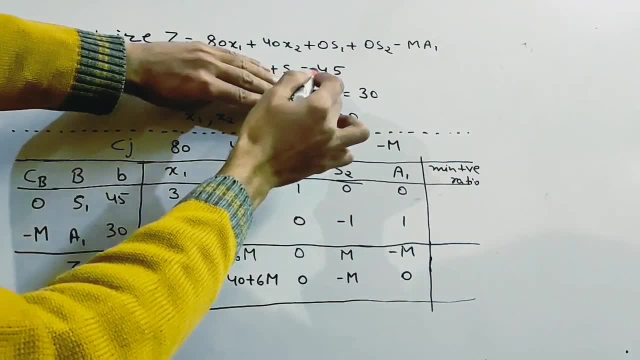 and A1.. What will be the values? S1 is equal to 45 and A1 is equal to 30.. And we have to keep these values as 0.. So what will be the values? S1 is equal to 45 and A1 is equal to 30.. 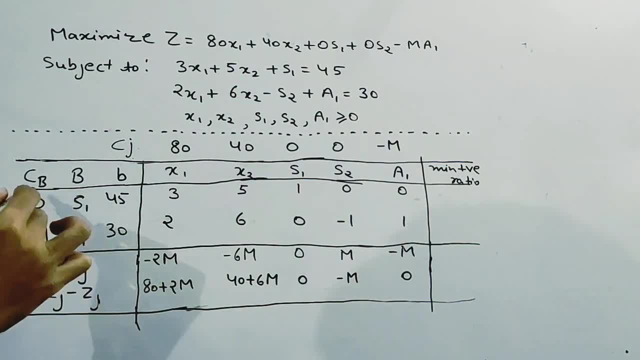 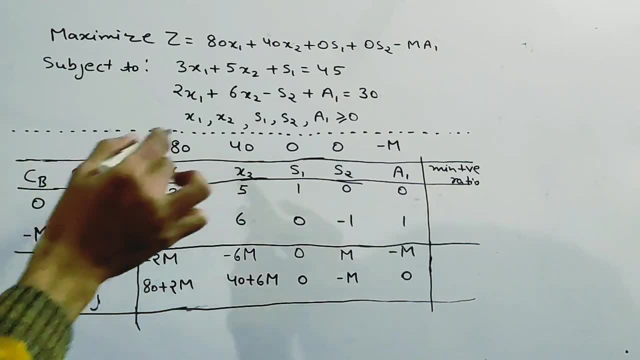 So what will be the values? S1 is equal to 45 and A1 is equal to 30.. Here we have noted down the coefficient in the objective function of these basic variables. S1's coefficient is 0, A1's coefficient is minus m. 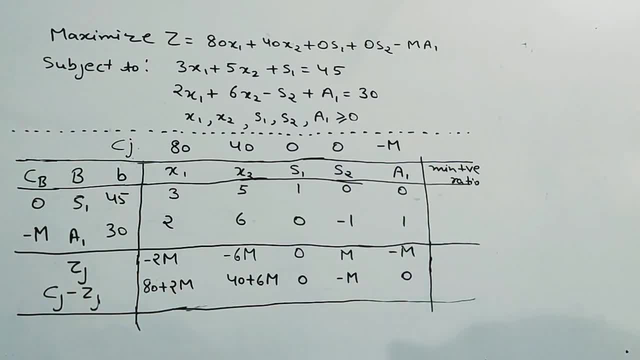 Then we have to see whether this solution is optimal or not. for that we need to calculate Zj value. Zj value, as I told earlier that it represents the outgoing profit or the amount of rate reduction in the objective function. How do we calculate Zj values? 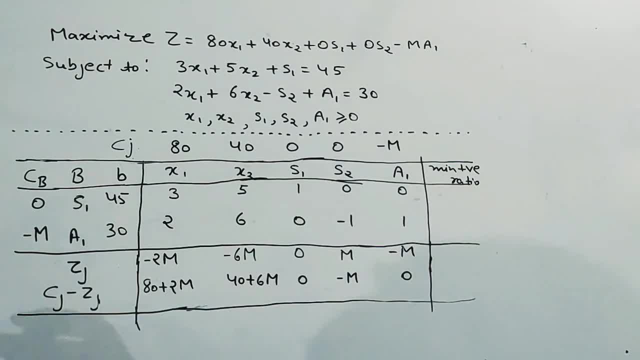 The Zj value of any column that we have to calculate, we have to multiply the corresponding Cb values of that column and add them. For example, 3 into 0 plus 2 into minus. m is equal to minus 2m, 5 into 0 minus 6m will. 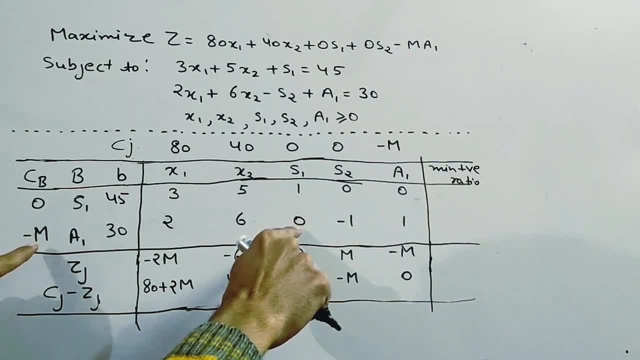 be minus 6m. 1 into 0 plus 0 into minus m is equal to minus 2m. 5 into 0 minus 6m will be minus 6m. 8 into minus m is equal to 0.. 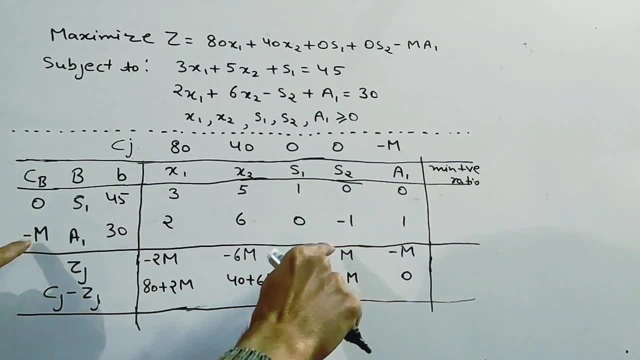 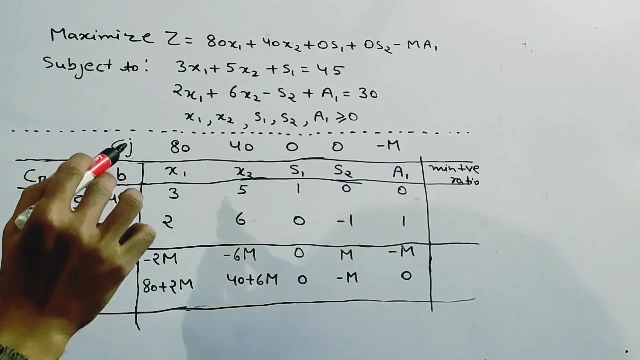 0 into 0, plus minus, 1 into minus m, which is plus m, and so on. Now we have to calculate Cj minus Zj values. Cj minus Zj values represent the net change in the objective function values, if any variable. 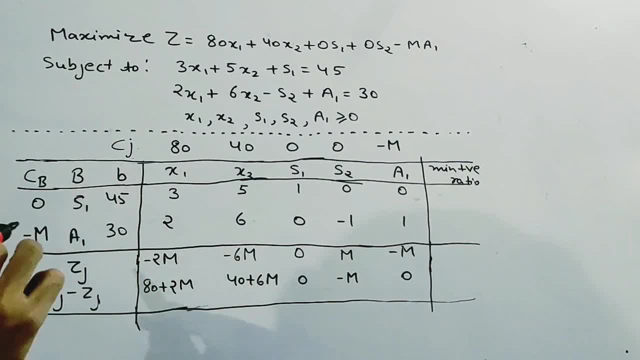 is introduced in the basis. Suppose if we produce one unit of X1, then it will be the addition of 80 rupees, while the minus 1 is zero. plus minus 1 is minus m, which is plus m minus 2m. reduction will happen. So net change will be 80 minus minus 2m, which is 80 plus 2m.